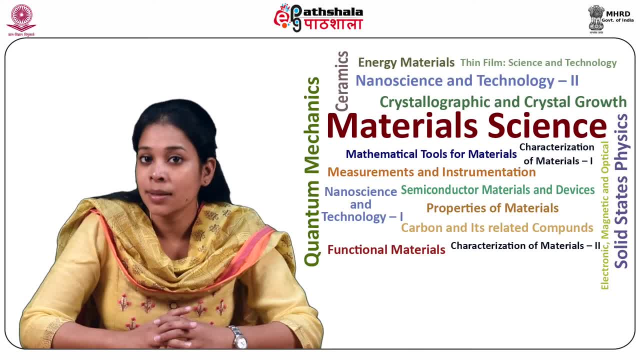 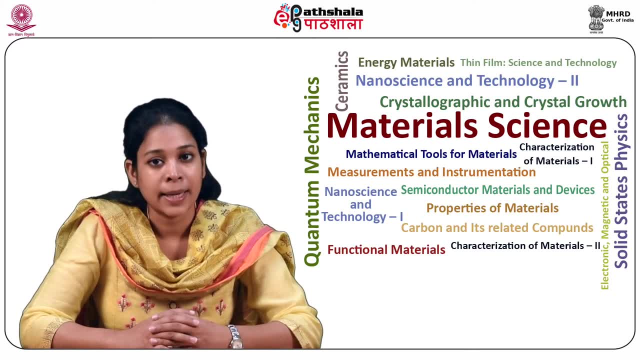 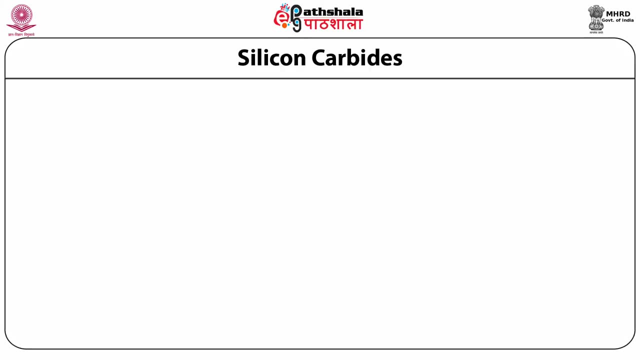 developed And in this module we will be discussing about these non-oxide structural ceramics, which are Silicon Carbide, Silicon Nitride, Cialons and newly developed MaX ceramics- Silicon Carbide- Silicon Carbide for application in plastic and hot healthy in refractories. we have already discussed in previous modules, So, as mentioned there, the two 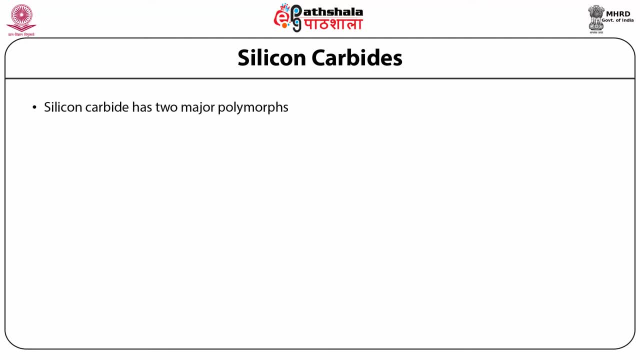 major polymorphs of silicon carbide are alpha silicon carbide, which has a hexagonal structure like woodzite, and beta silicon carbide, which has a zinc blend structure like diamond. Of the two, the alpha phase is marginally more stable than beta polymorph because of its low 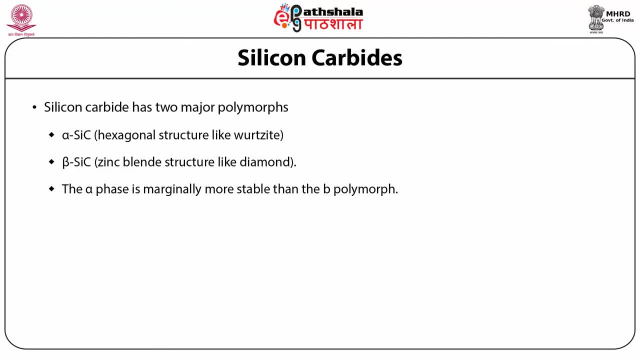 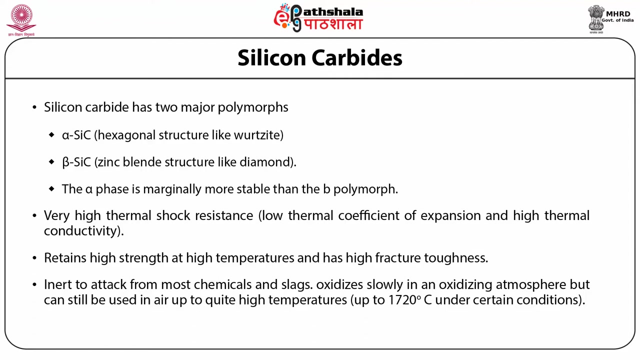 thermal coefficient of expansion and high thermal conductivity. it has a very high thermal shock resistance. It retains high strength at high temperatures and has high fracture toughness. It is inert to attack from most chemicals and slags. It oxidizes slowly in an oxidizing atmosphere but can still be used in air up to 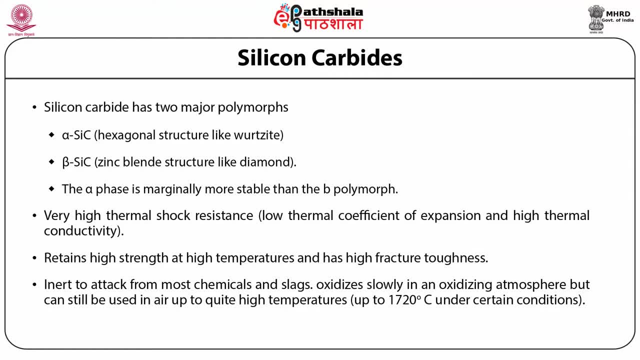 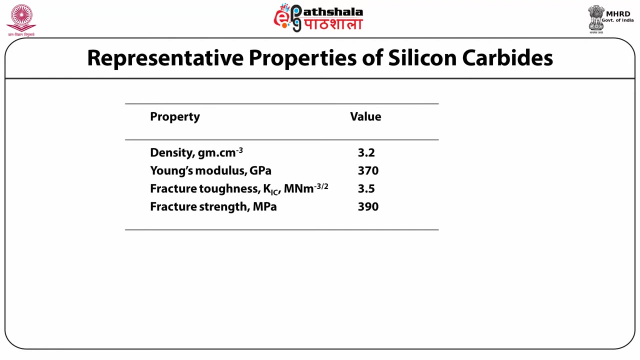 quite high temperatures, that is, up to 1720 degree Celsius under certain conditions, and almost up to its dissociation temperature, that is, 2400 to 2700 degree Celsius in the inert atmosphere. So, students, you can see the representative properties of silicon carbide and you can see that the 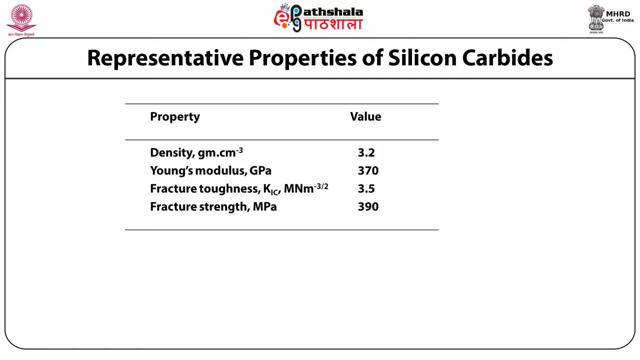 density of silicon carbide is 3.2 gram per centimeter cube. The Young's modulus is 370 gigapascal. The fracture toughness is 3.5 mega newton meter to power minus 3 by 2.. Whereas the fracture strength is 390 mega pascal. 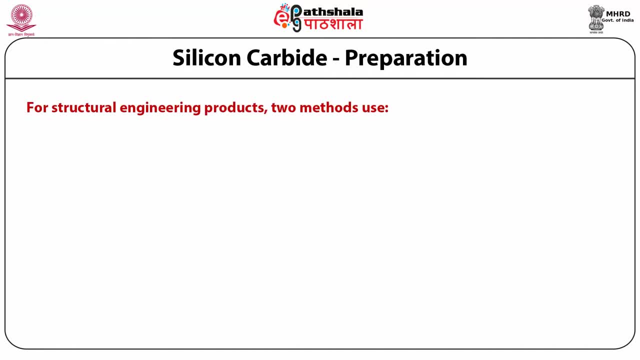 Silicon carbide preparation. So for application and structural engineering products, silicon carbide bodies are fabricated through two routes. So the first is reaction bonding and the second one is centering of ultra fine powder with some dopants. In reaction bonding or reaction sintering, a mixture of silicon carbide and carbon are compacted and infiltrated. 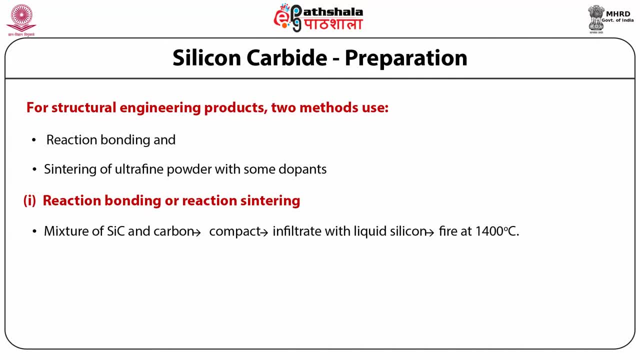 with liquid silicon. Firing is carried out at 1400 degrees Celsius. Silicon and carbon react to form beta silicon carbide, which bonds the pre-existing silicon carbide grains. It is difficult to react the silicon totally. About 8-10% silicon remains unreacted because of 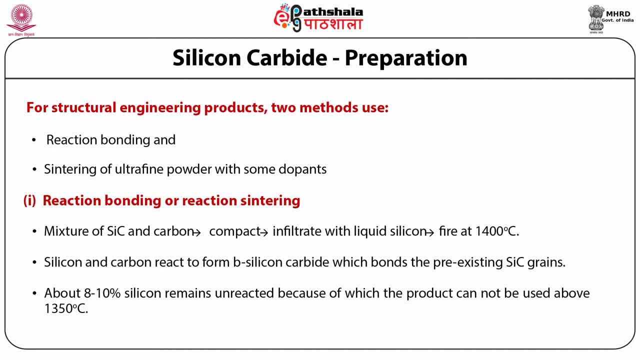 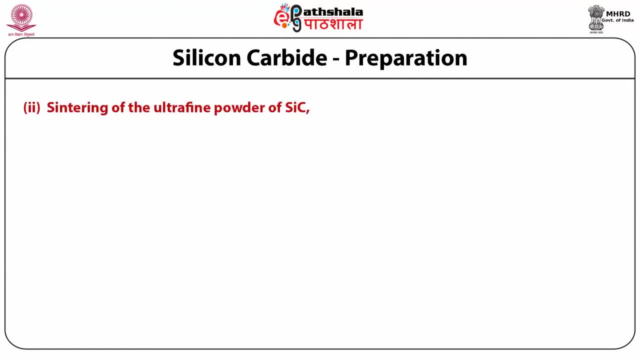 which the product cannot be used above 1350 degrees Celsius. In the sintering of ultrafine powder of silicon carbide, the additives like carbon and boron or carbon and aluminium are used. Dopens like iron, lithium and magnesium are also used. The dopens are so selected that they do not 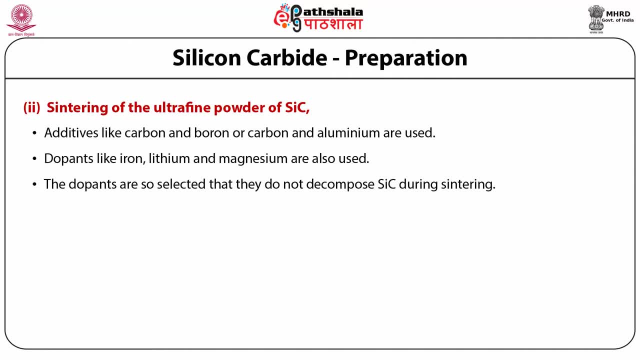 decompose silicon carbide during sintering. The carbon plays an important role during the sintering of silicon carbide. It increases the concentration of point defects, which increases the diffusion. It increases the concentration of point defects, which increases the diffusion. It increases the 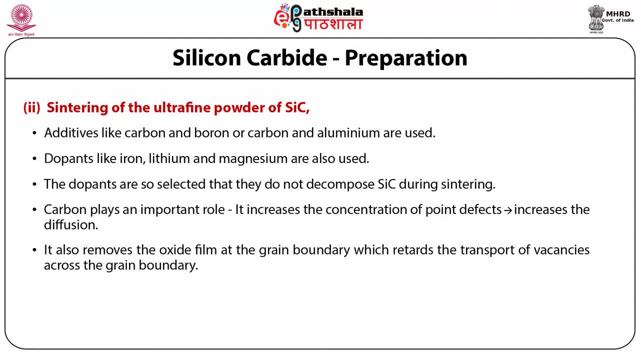 concentration of point defects, which increases the diffusion. It also removes the oxide film at the grain boundary, which retards the transport of vacancies across the grain boundary. The compact is sintered in an inert atmosphere between 2000 to 2100 degrees Celsius and a complex set of 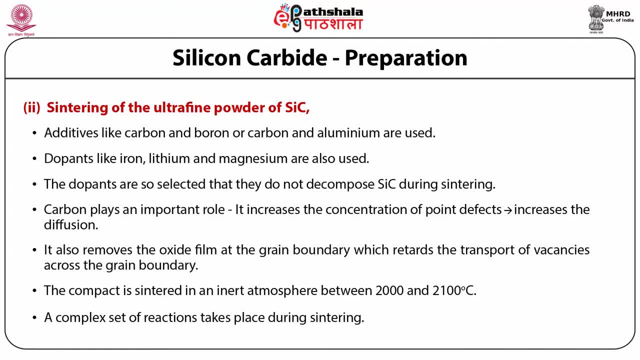 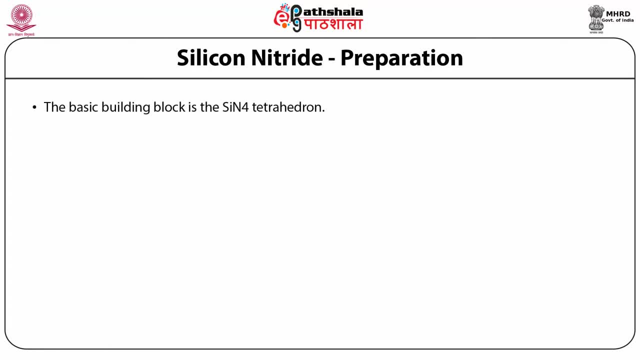 reactions takes place during sintering. Now here comes silicon nitride and its concentration. The basic building block of the structure of silicon nitride is sin4 tetrahedron. The tetrahedra are linked at the corners. The silicon nitride bond are short and they are very strong. 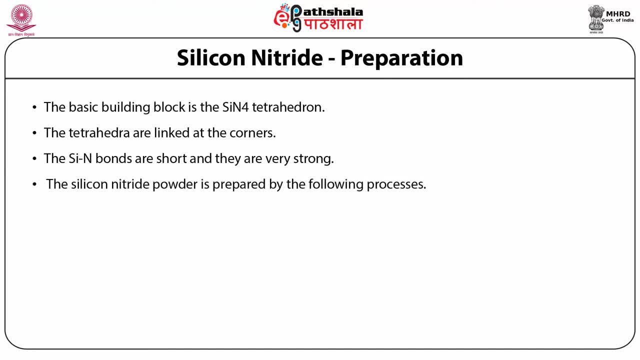 The silicon nitride powder is prepared by the following process, which we will discuss one by one. So the first is direct nitridation, The second is direct nitridation of silicon. This is the method most used in commercial practice and the following reaction occurs: like 3Si plus 2N2 gives Si3N4. Here delta H is minus 175 kilocalories per mole. 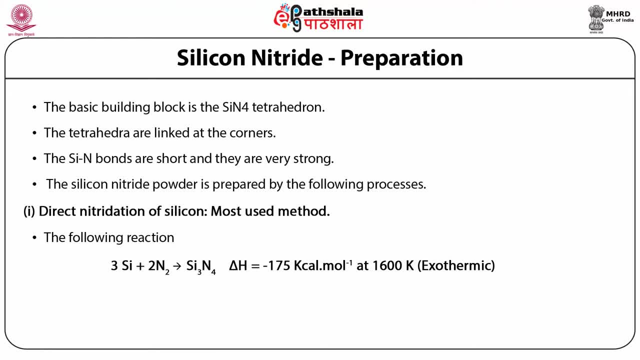 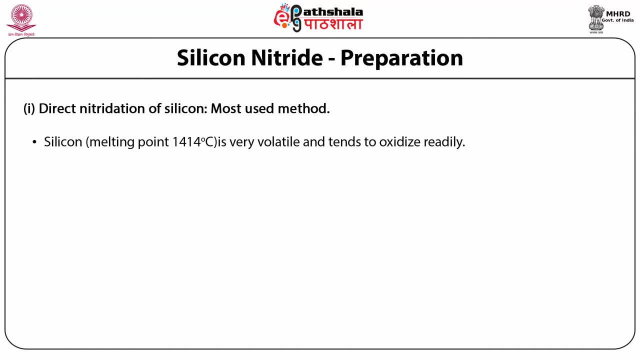 at 1600 Kelvin, so it is exothermic. The melting point of silicon is 1414 degrees Celsius And the silicon is very volatile at temperatures near the melting point. Also, it tends to oxidise readily and on the other hand, complete nitriding is not possible unless the 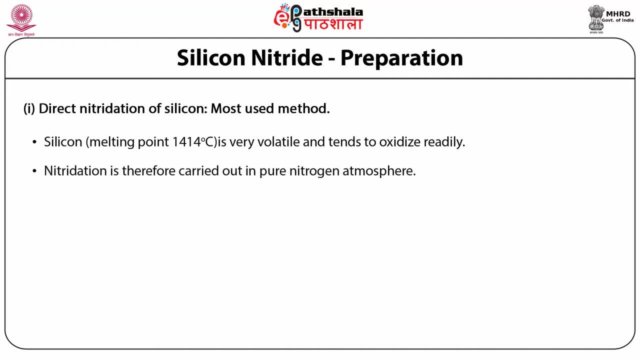 silicon is melted. The nitriding is therefore carried out in pure nitrogen atmosphere, so to reduce the silicon volatilization. the reaction is carried out in two stages, that is, for 25 to 50 hours at 1325 to 1350 degree celsius, followed by 10 to 25 hours at 1425 to 1450 degree celsius. 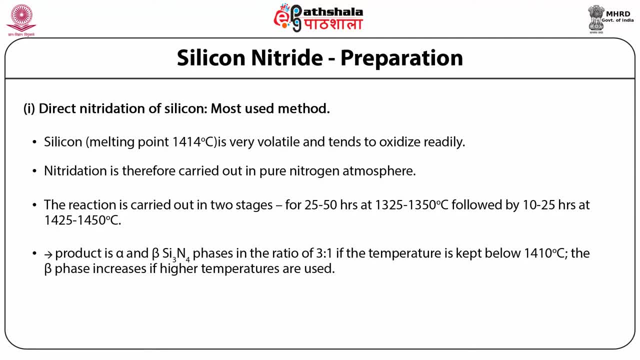 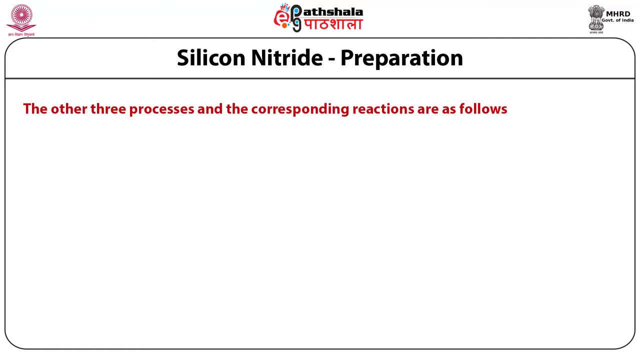 The product consists of alpha and beta silicon nitride phases in the ratio of 3 to 1 if the temperature is kept below 1410 degree celsius, whereas the beta phase increases if the temperatures are used. The other three processes and the corresponding reactions are as follows. 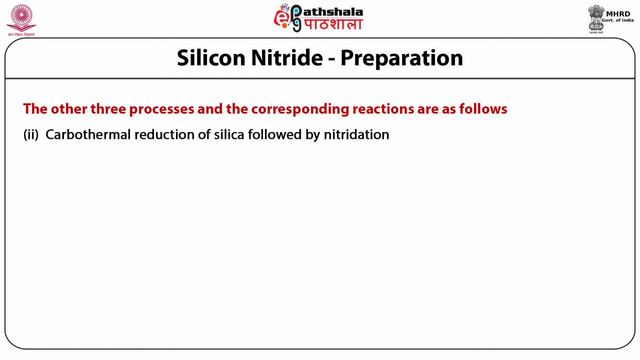 So the next one is Carbothermal reduction of silica, followed by nitridesion. In this case the reaction is 3SiO2 plus 6C plus 2N2 gives Si3N4 plus 6CO. So here delta H is 303 kilocalories per mole. 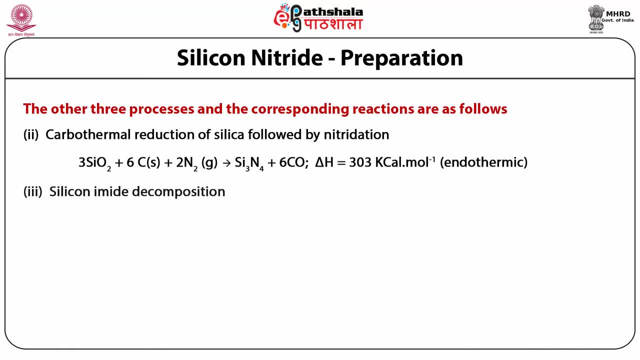 which is endothermic. The next is silicon imide decomposition. So in this the reaction is: SiCl4 plus 6NH2 gives SiNH whole twice plus 4 times NH4Cl at room temperature, and then 3SiNH whole twice gives Si3NH4 plus 2NH3 at 1200 to 1500 degree celsius. The next phase is gas phase synthesis. 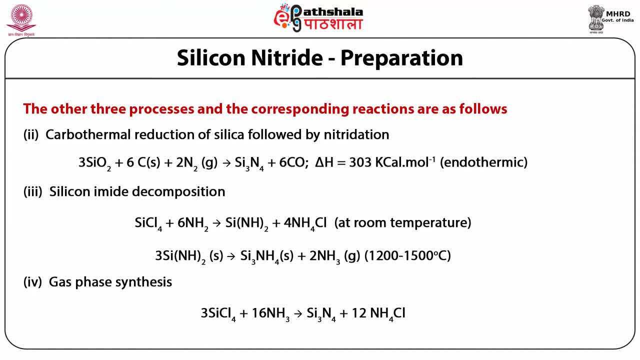 in this 3SiCl4 plus 6C plus 2NH3 at room temperature. So in this case the reaction is 3SiCl4 plus 6C plus 2NH3 at room temperature. 16NH3 gives Si3N4 plus 12NH4Cl to prepare sintered silicon nitride body. several methods: 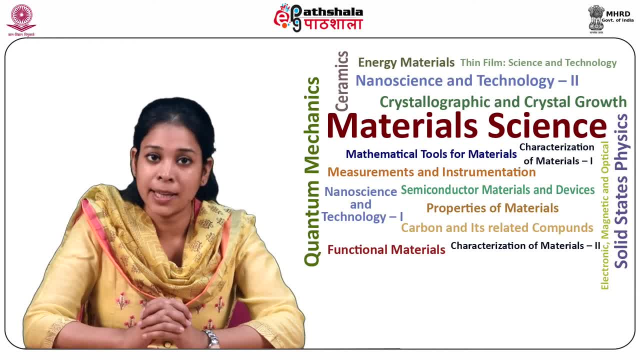 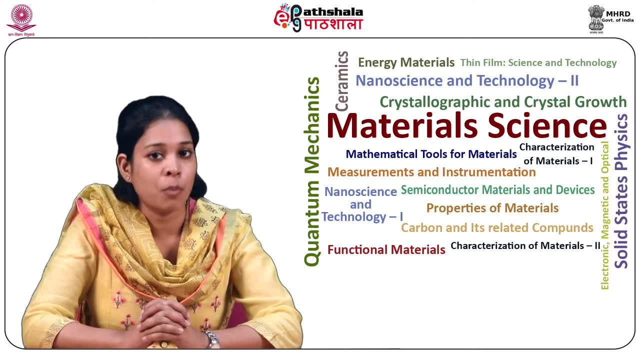 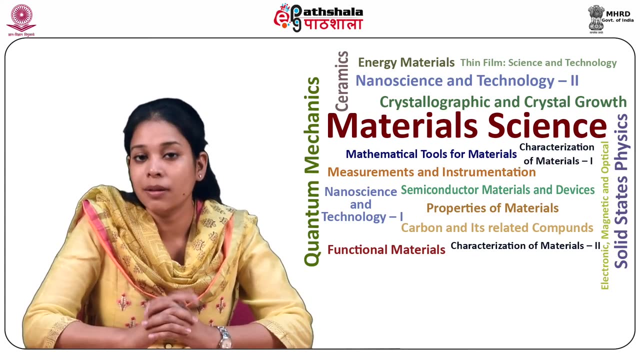 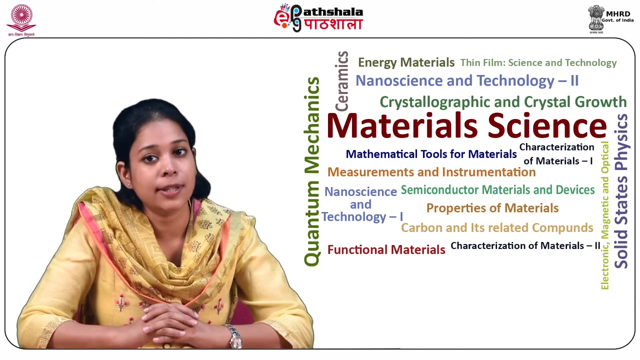 are used depending on the application. So let us discuss these methods one by one. So the first is reaction bonding or reaction sintering. In this process, the silicon powder is compacted into a desired shape. It is heated to 1200 degree Celsius in an atmosphere of nitrogen. 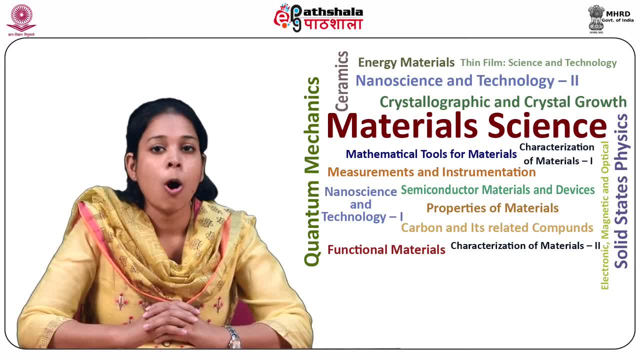 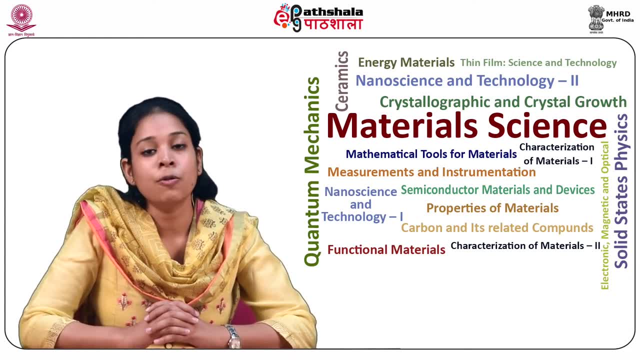 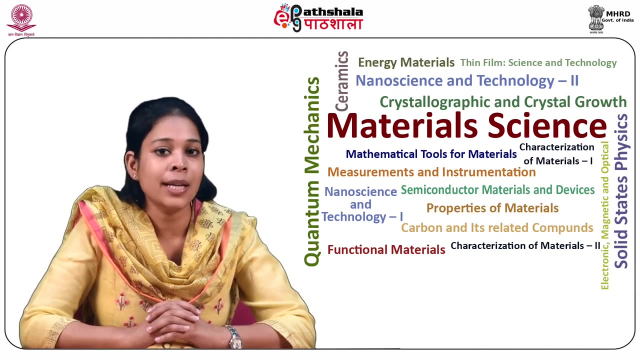 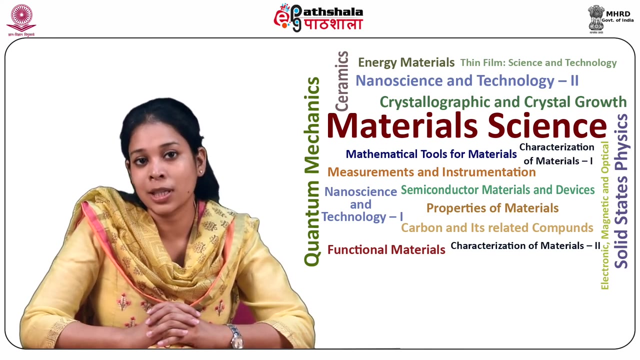 or mixture of nitrogen and hydrogen, or it can be nitrogen and argon, So the nitrogen reacts with silicon to form silicon nitride. So initially alpha silicon nitride fibers grow into the pores of the compact. Then the temperature is gradually raised to 1400 degree Celsius, and now mostly 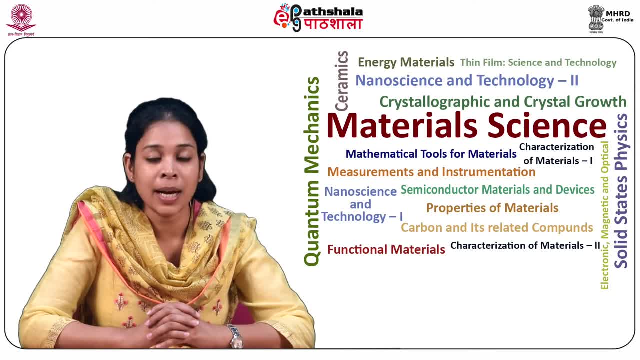 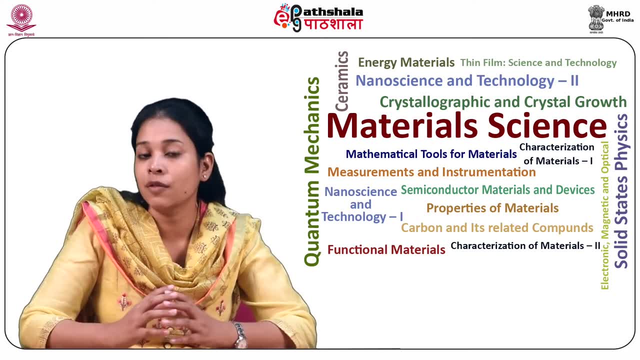 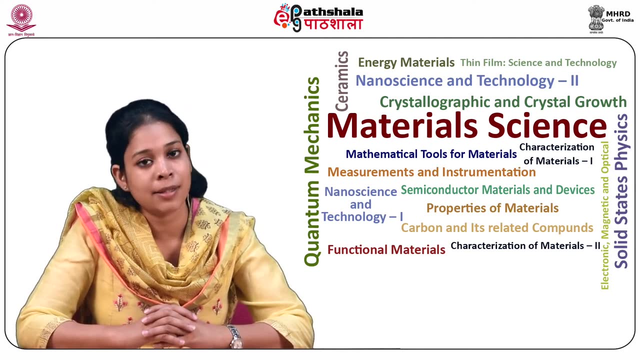 beta silicon nitride, that is beta Si3N4 forms. So the density of about 85 percent is achieved and the final microstructures consist of grains of alpha and beta phases. So the hot pressed silicon nitride fibers grow into the pores of the compact. So the temperature is gradually raised. 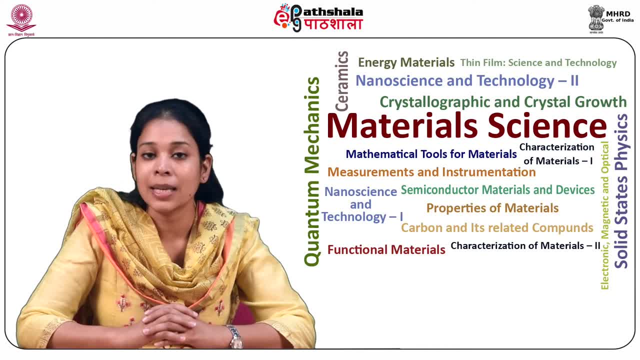 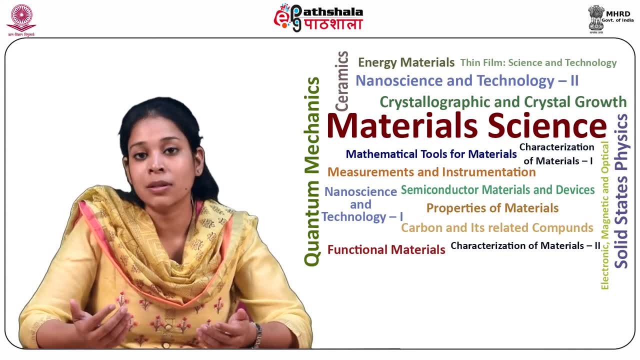 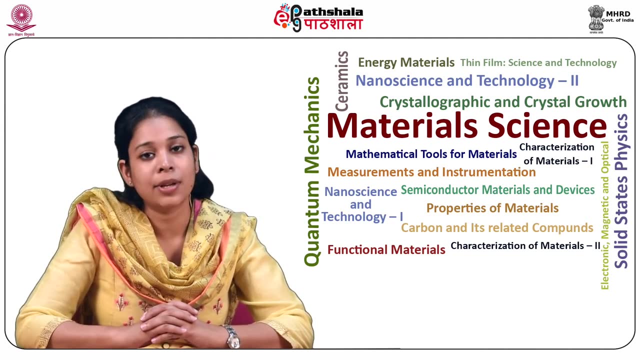 to 1200 degree Celsius in an atmosphere of nitrogen and nitrogen also forms. So the definition is that the high density silicon nitride is the next procedure, that is HPSN. So in this technique the silicon nitride powder is mixed with some additives and hot pressed at 1700 to 2000 degree Celsius. 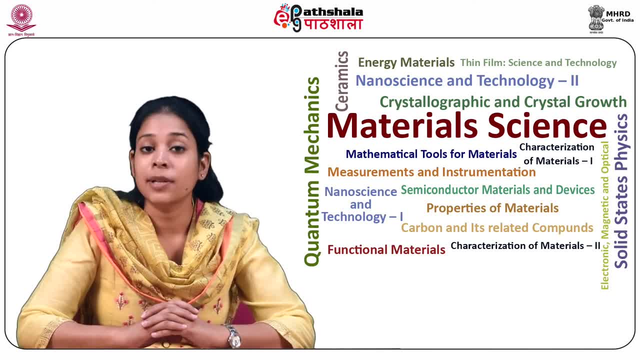 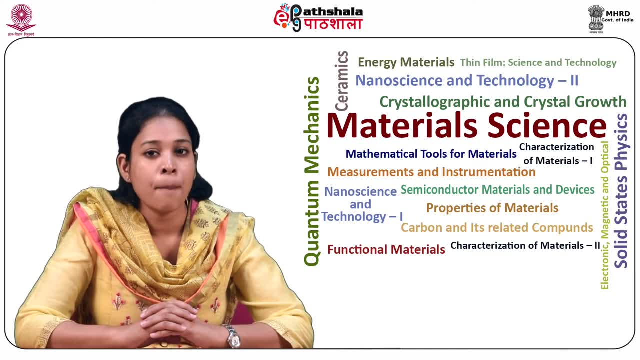 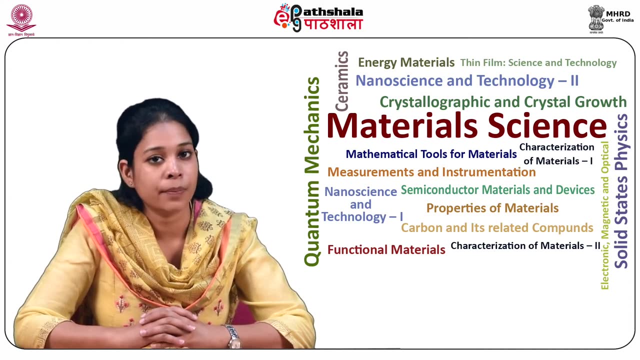 So the hot pressing produces simple shapes. Very high densities and strengths can be achieved using this technique, but for the high density silicon nitride the preference is to use silicon nitride. complicated shapes: the hot isostatic pressing is usually used. Now the next is liquid phase. 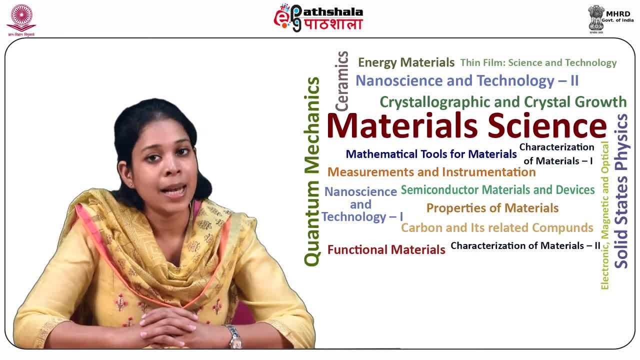 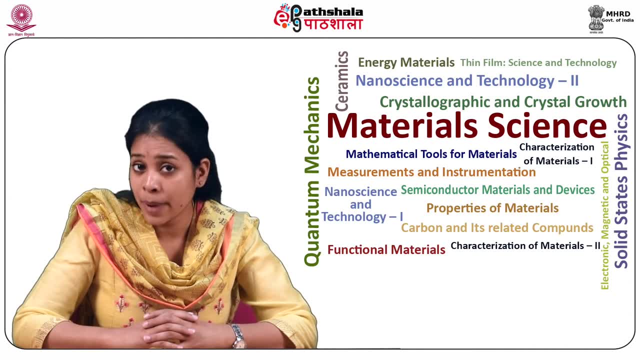 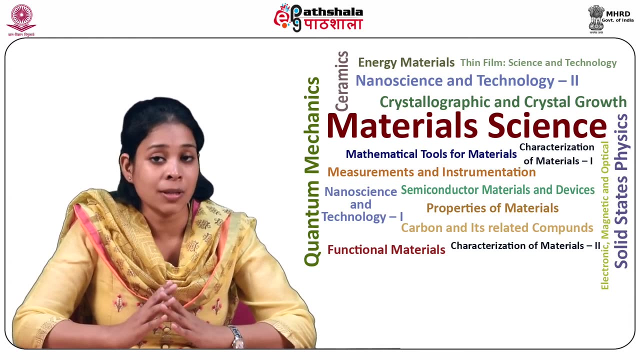 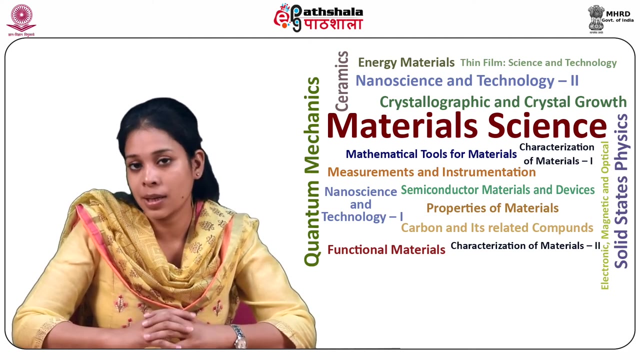 sintered silicon nitride, that is LPSSN. So the large amount of suitable additives and the silicon nitride powder is used to carry out the liquid phase sintering. So an inexpensive process is liquid phase sintered silicon nitride, which yields adequate properties suitable for many. 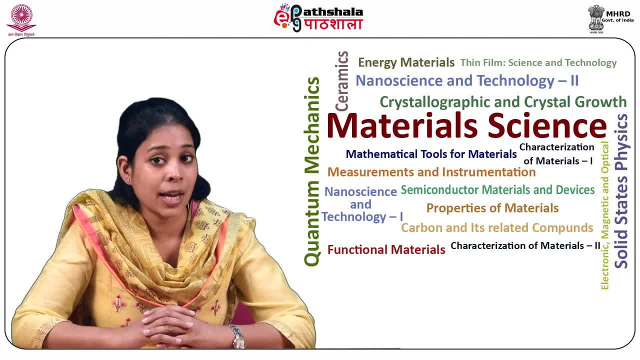 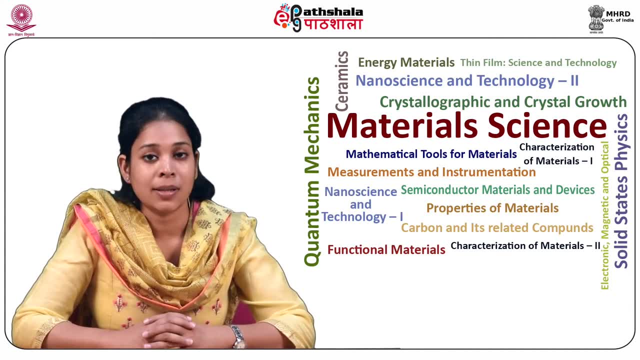 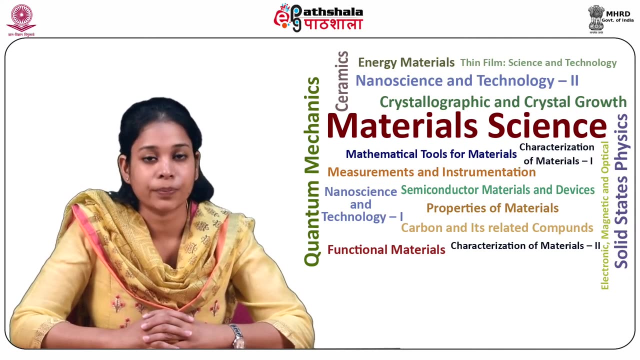 applications. So a large number of sintering aids are used to sinter the silicon nitride, and some of these are uterium oxide, that is Y2O3, or magnesium oxide, that is MgO. Now the next is gas pressure sintering. 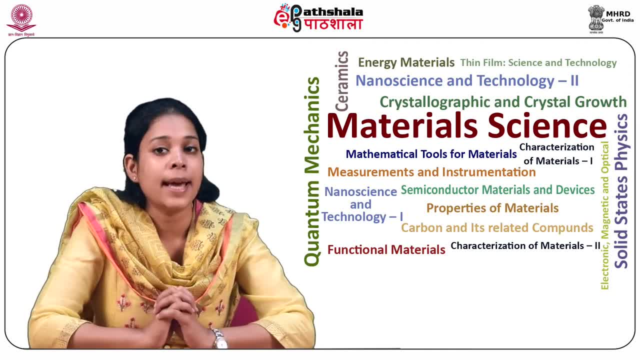 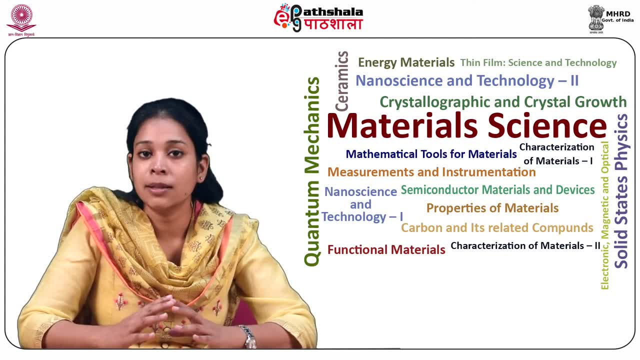 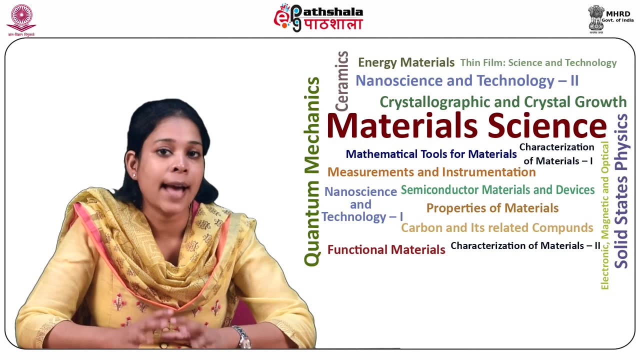 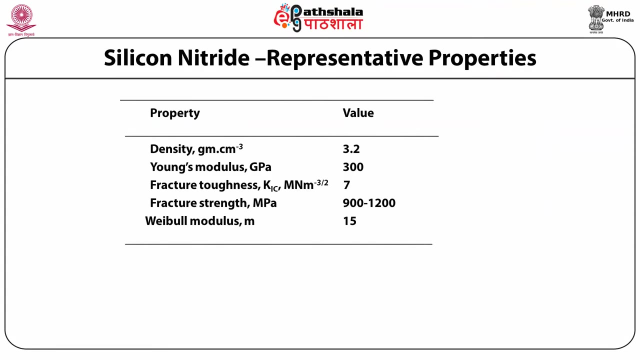 So in this process the silicon nitride powder with sintering aids is sintered at a high pressure, but a high nitrogen pressure is used. So in this technique a gas is used. that's why the name is gas pressure assisted sintering technique. So the representative properties of silicon nitrides. 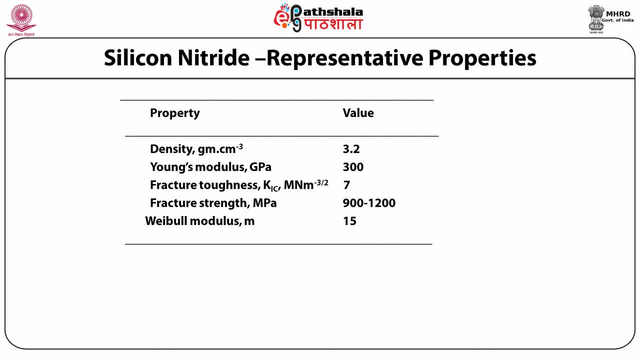 are tabulated in this table: Guidelines geworden. gas pressure. Coagulated gas pressure. It is aimed at reducing the number of siolianes. breast size, 뚫 Density is 3.2 gm. idols is 300. gigapascal fractured toughness: 7,. ciolons is 700. scalars é. 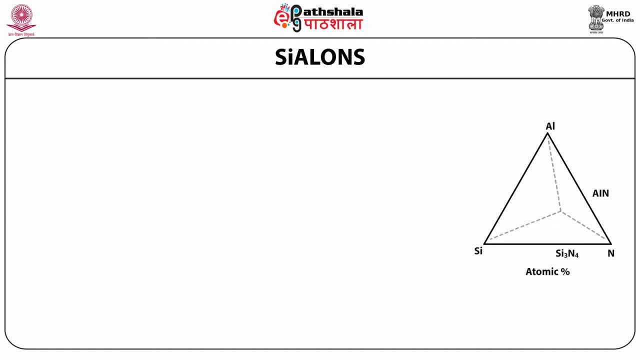 So that the density of silicon nitride is 3.2 g per centimeter to Young's models is 300 giga. Pascal Fracture otress: 7 m M Minus 3 by two fractures. Minus 3 by 2 fractures, strength is 900 to 1200 mega Pascal. webinar modulus is 15 meters. 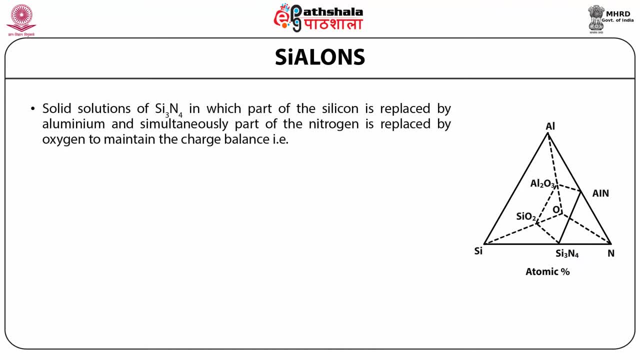 CR loans. CL ons arre the, so I would solutionThank you for your attention to this Request-uckbookcom with Asia Lewis Hewitt, Our он and yeah of silicon nitride, that is, Si3 and 4, in which part of silicon is replaced by aluminium, and. 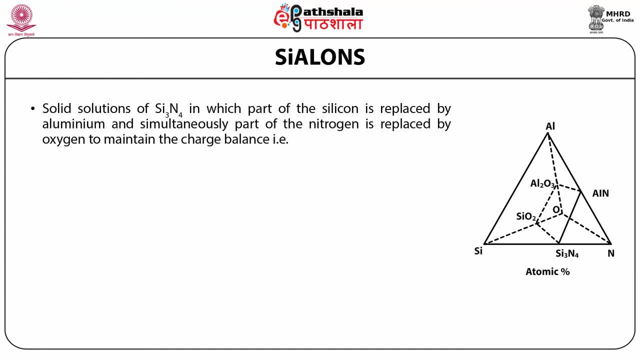 simultaneously, part of nitrogen is replaced by oxygen to maintain the charge neutrality. that is in silicon nitride. Si is Si plus aluminium and nitrogen is nitrogen plus oxygen. So they can be looked upon as a part of the quaternary system, that is, SiO2, Si3N4, AlN, Al2O3.. So there are 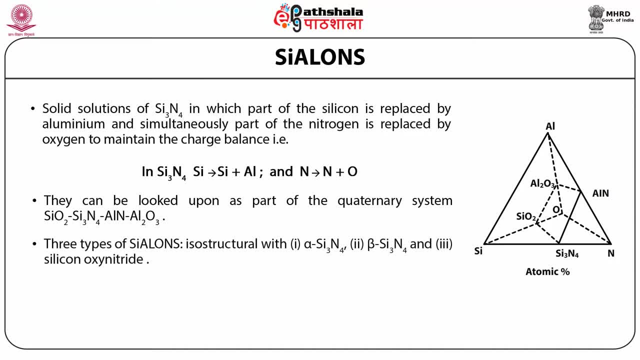 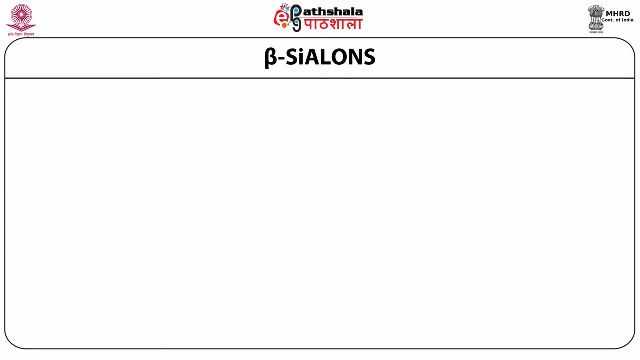 three types of C-alons: with isostructural, with alpha Si3N4,, beta Si3N4 and silicon oxynitride. So the most common are beta C-alons which have the general formula Si6-nitride, Si6-z, Alz, Oz, N 8-z. So beta C-alons are the most commonly used and they have the general 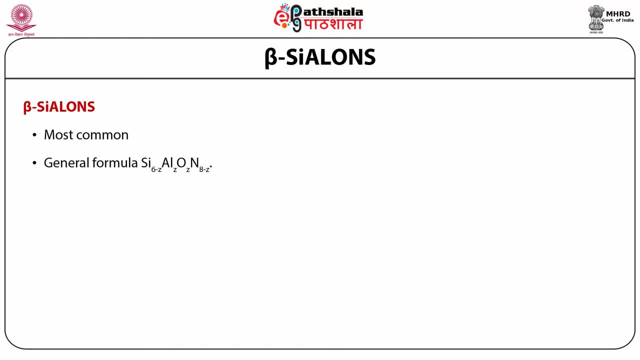 formula which we have discussed in the previous slide is Si6-z- Alz Oz- N 8-z. So the sintering aids, such as the yttrium oxide, that is, Y2O3, or Si6-z- Alz Oz- N 8-z. So beta C-alons are the most commonly used and they have the general formula which we have discussed in the previous slide, is Si6-z, Alz, Oz, N 8-z. So the sintering aids, such as the yttrium oxide, that is Si6-z, Alz, Oz, N 8-z, So beta C-alons are the most commonly used and they have the general formula which we have discussed in the previous slide, is Si6-z, Alz, Oz, N 8-z. So the sintering 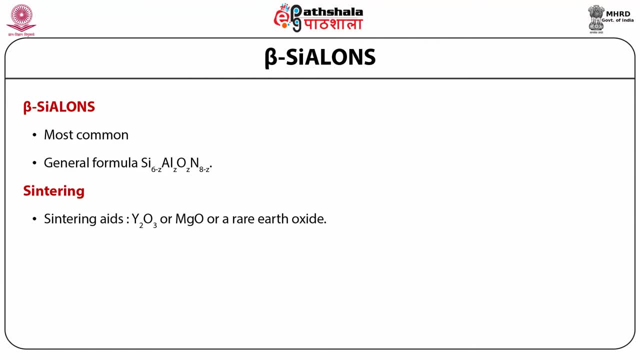 that is MgO or a rare earth oxides are used to densify. More liquid is formed at lower temperatures than in the case of silicon nitride, and the densification is better On sintering above 1700 degree Celsius. the elongated hexagonal beta cellulons grain grow in an oxynitride liquid phase. 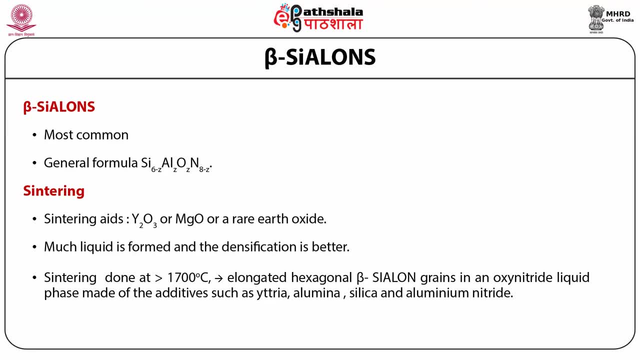 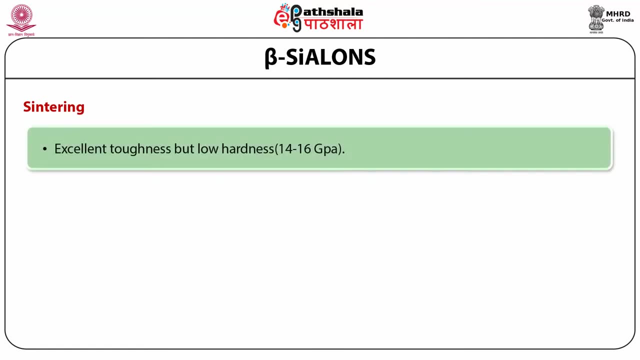 made up of additives such as yttria, alumina, silica and aluminium nitride. The liquid phase forms a high temperature glass on cooling. So the beta cellulons have excellent toughness, but their hardness, which is 14 to 16 gigapascal, is low. The alpha cellulons have higher hardness. 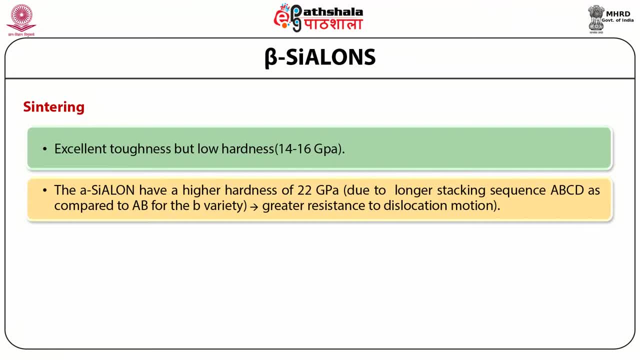 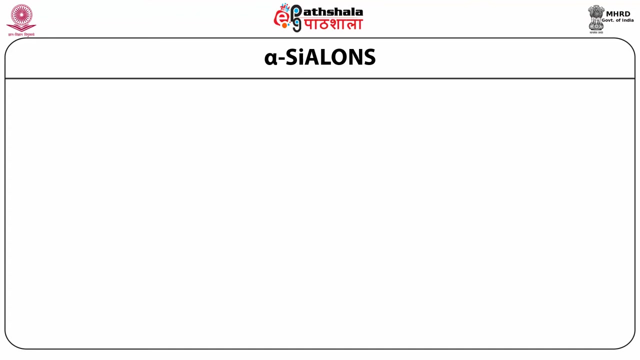 of 22 gigapascal and this comes from their longer stacking sequence, that is, ABCD as compared to AB for the beta variety. So such a structure provides a high resistance to dislocation motion. Alpha cellulons- The alpha cellulon materials produced earlier- had a microstructure of fine equi-egged grains. Consequently, 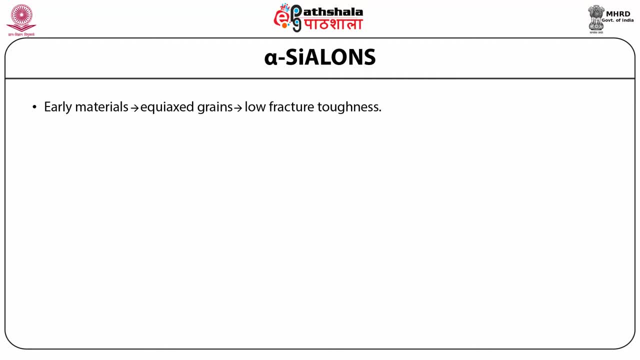 the material had a low toughness. over the years, Progress has been made to produce a microstructure with interlocking and elongated grains. this has resulted in a surface los material of high fracture toughness. in alpha cellulon It is essentially a solid solution of alpha SI3 and 4 in which there is a Standard. 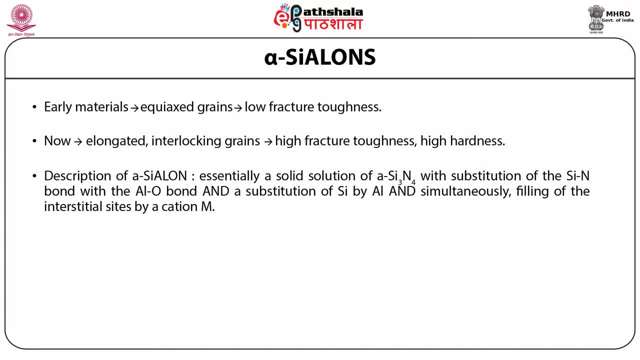 Substitution of alpha si 3 and 4, in which there is a Standard Substitution of alpha Si3 & 4 of Alpha si3N4.. In alpha sea linear- So so thin and weak You can saw theuje- the silicon nitride bond with the aluminium oxide bond. In addition, there is substitution of: 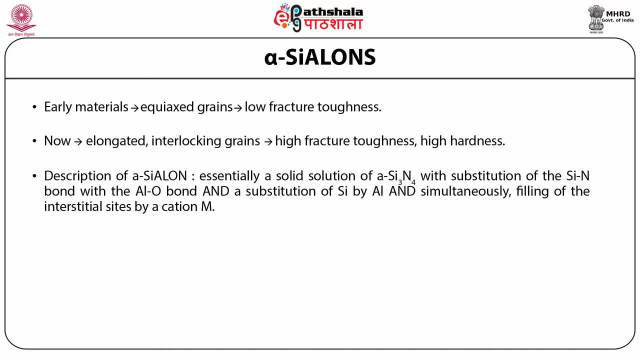 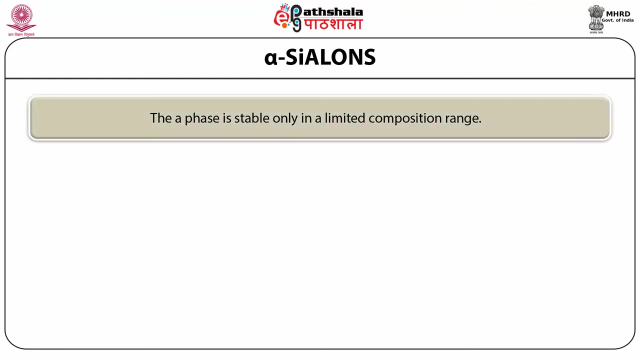 silicon by aluminium and simultaneously filling of the interstitial sites by a cation, M. It has a general formula that is: M, M by Z, SI 12 minus M plus N, AL, M plus N, ON, N 16 minus N, where M is the interstitial cation with a valence or Z. The alpha phase is stable only in a limited. 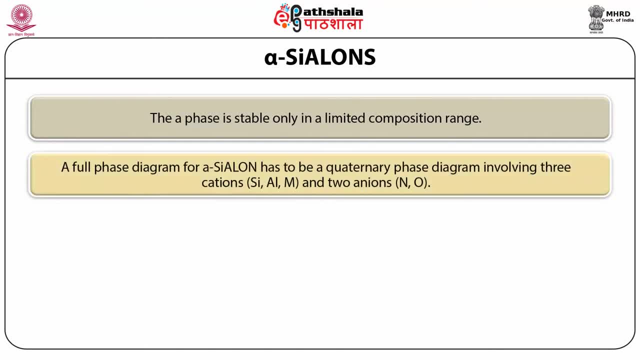 composition range. A full phase diagram for alpha cation is. a full phase diagram for alpha cation has to be quaternary phase diagram involving three cations, that is, silicon, aluminium and M, and two anions, that is, nitrogen and oxygen. However, a binary phase diagram may be used to. 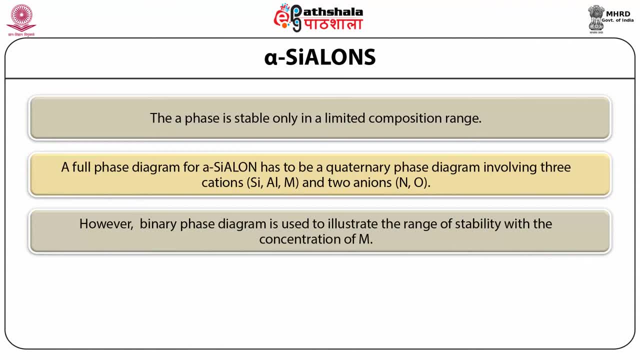 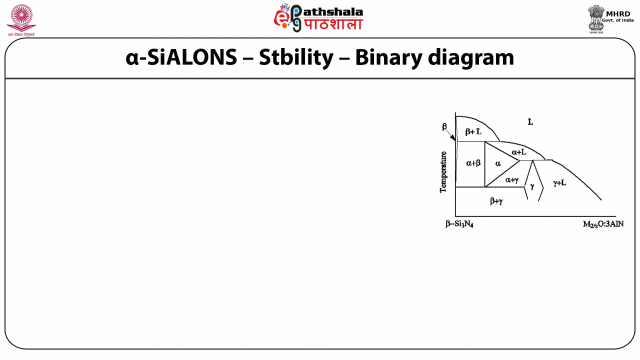 illustrate the range of stability with the concentration of M. Such binary diagram is between silicon nitride, that is, silicon and M. So, students, you can see a figure on the top left corner of the slide showing the pseudo-binary phase diagram between beta silicon nitride, that is, Z and M. 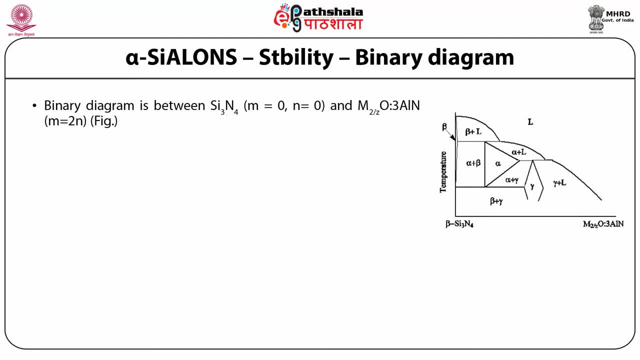 Beta, SI 3 and 4 and M 2 by Z O is to 3 aluminium nitride, showing the region of stability of the alpha C-ALON phase. So in the figure you can see that the horizontal composition line in this 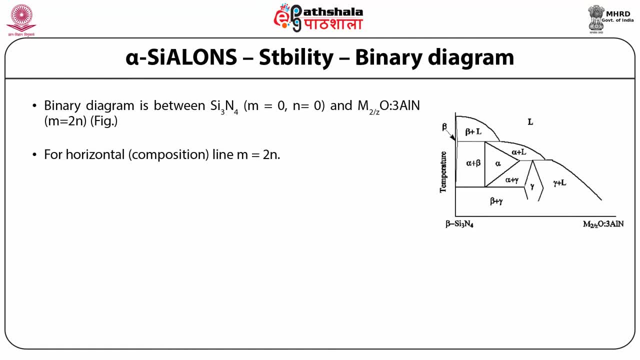 diagram correspond to M is equal to 2N. In this phase diagram, the alpha C-ALON exists as a eutectoid phase and its phase diagram corresponds to: M is equal to 2N. So in this phase diagram, 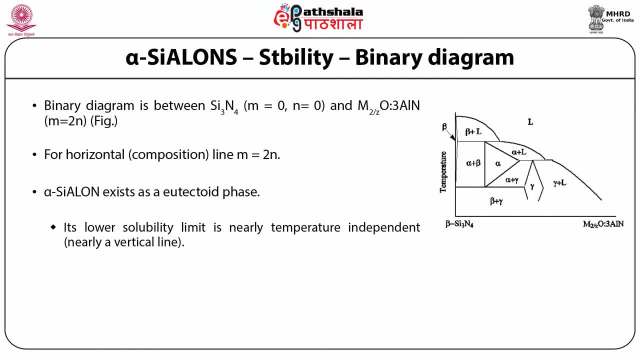 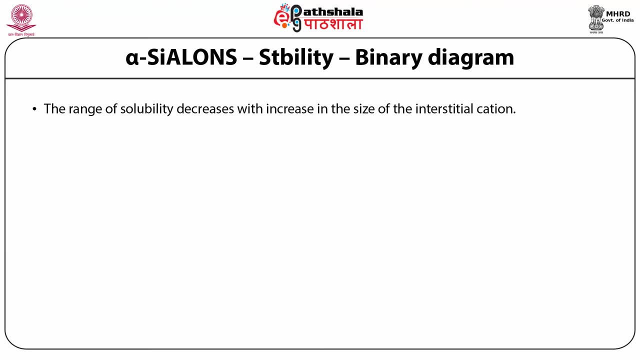 we have observed characteristics of the partial site and its partial margins in one strain, Say B singing 1. the integer of the output in duck holes is integral to Amazon outbreaks and O is fruits of domestic Corona, where it decreases as the size of the interstitial cations decreases. 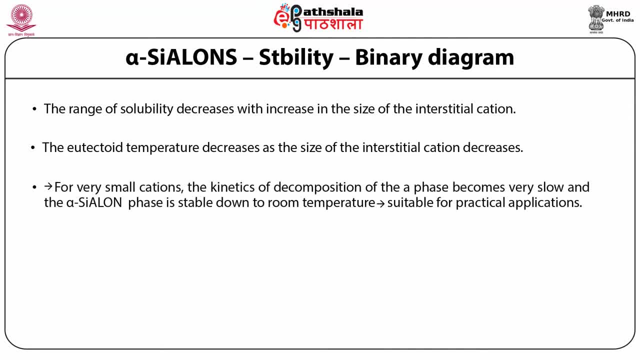 It becomes so low for small cations that the kinetics of the decomposition of the alpha phase become very slow. and the alpha Ceylon phase is stable down to room temperature. This material is suitable for the practical applications. The region of stability of the alpha Ceylon expands with decreasing size of interstitial 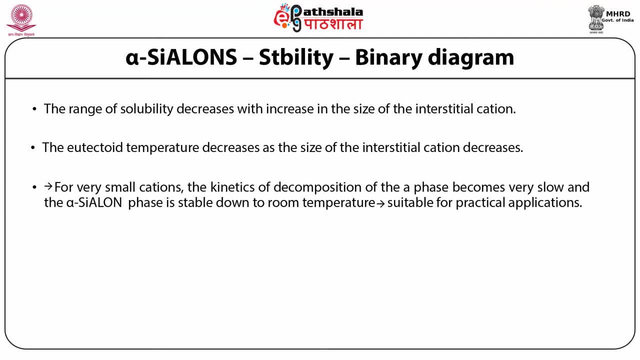 cation M. Thus, when the interstitial cation M is equal to Nd, the stability region of alpha Ceylon is very small. In this case, the alpha Ceylon decomposes when held in a particular temperature range, So the particular temperature range is very small. 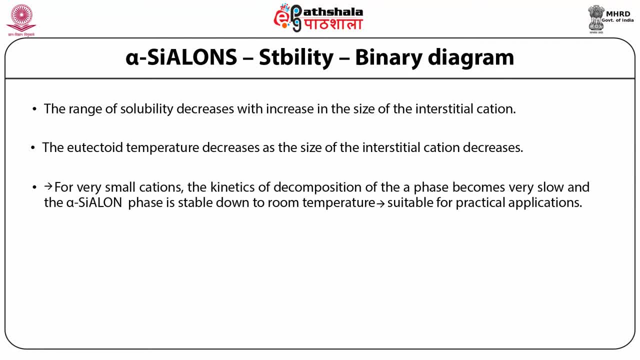 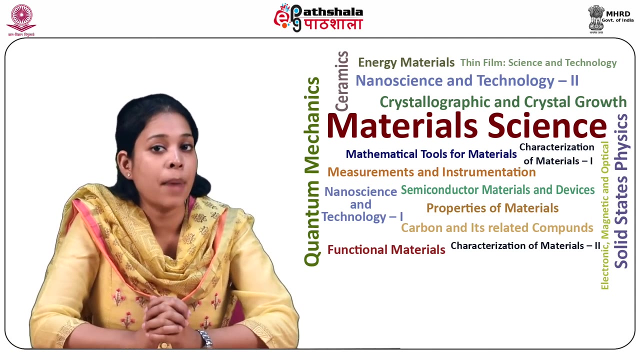 The particular temperature range will be 1400 to 1500 degree Celsius. The stability region is quite large for yttrium and by B, and so these alpha Ceylons are stable in the useful temperature range. Initially, the alpha Ceylon ceramics were fabricated using powders having more than 90% of alpha. 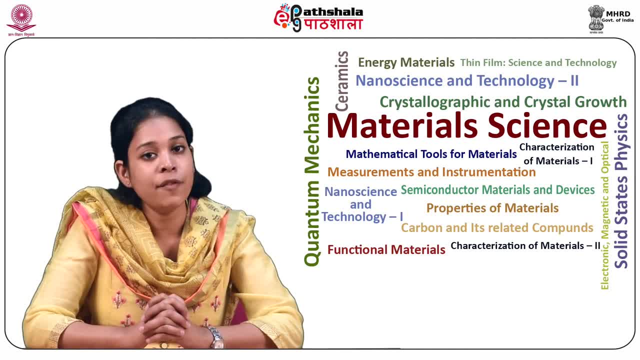 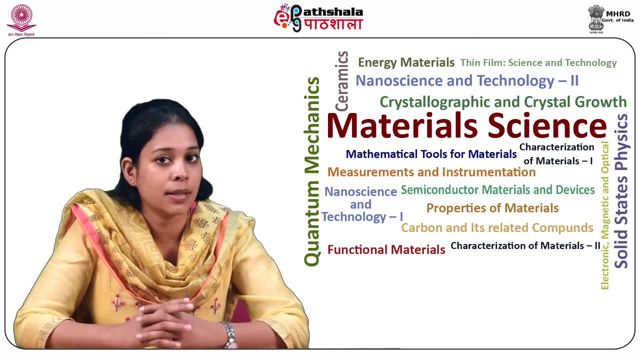 silicon. However, the alpha Ceylon ceramics were made using the same matrix of nitrites ie, si3N4, and these particles provided the nucleation sites for alpha Ceylon's grains. This produced an equiaque structure of alpha Ceylon and this material had a high strength. 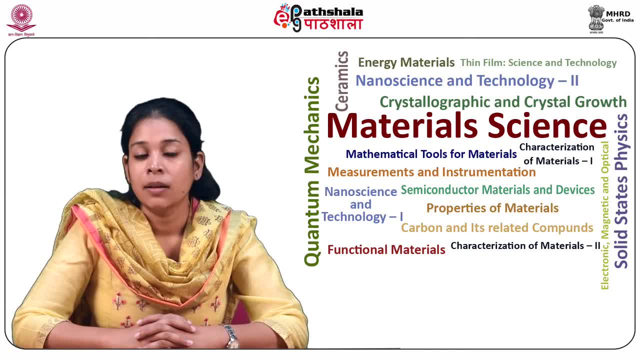 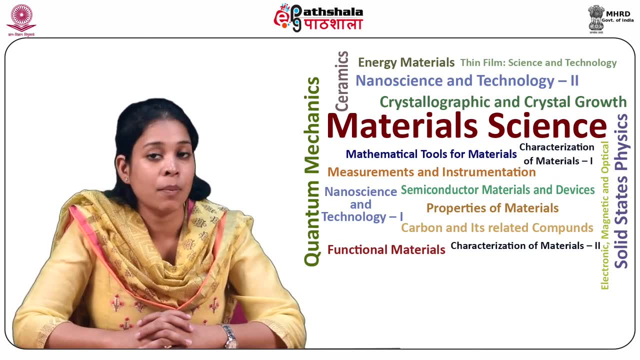 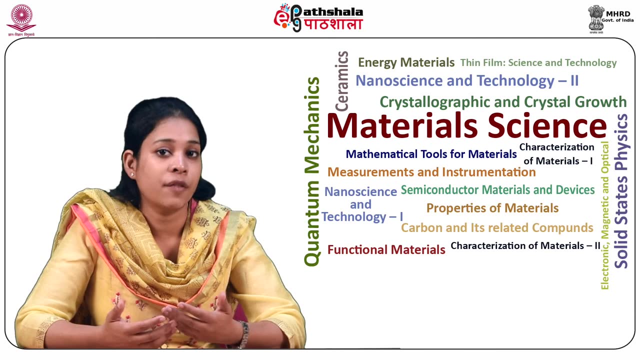 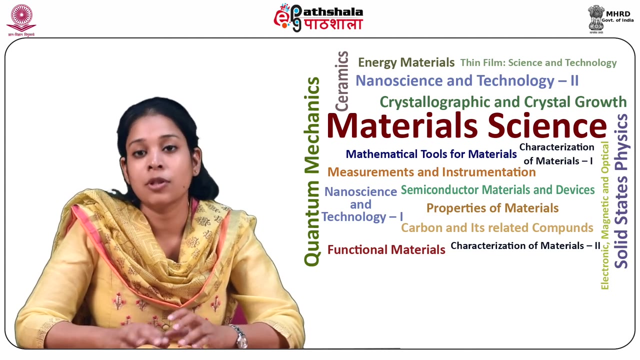 but low fracture toughness. So the key to produce alpha Ceylon ceramics with elongated grains status to improve the prove the fracture toughness, is to have very few nuclei for the formation of alpha coelons in the starting powder and during the heating and forming steps. this procedure is taken. 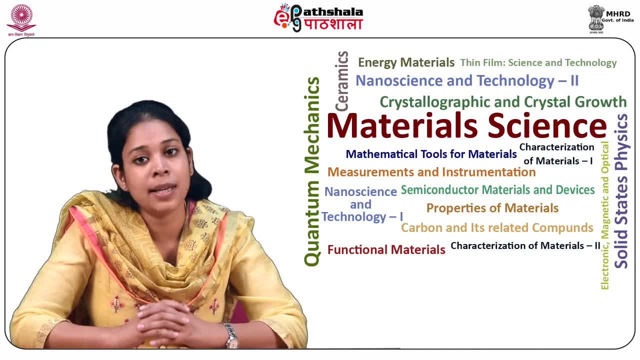 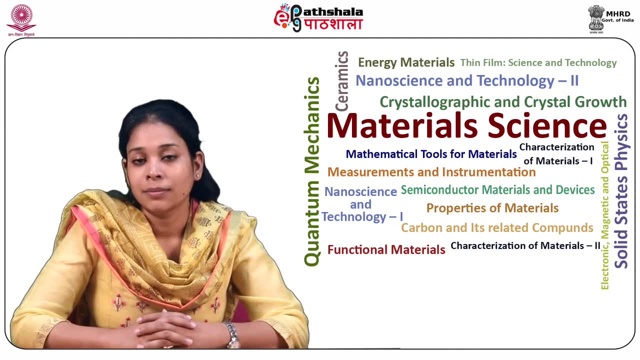 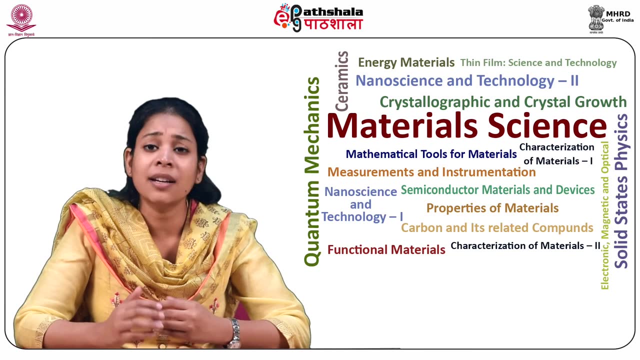 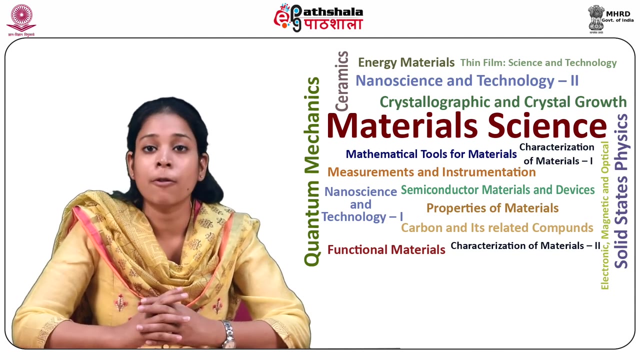 care. So it has been found that alpha coelon can be produced by starting from beta silicon nitride, that is, beta Si3N4, and rare earths in the starting powders. Thus, in most compositions for which the stability of alpha coelon phase is low, the proportion. 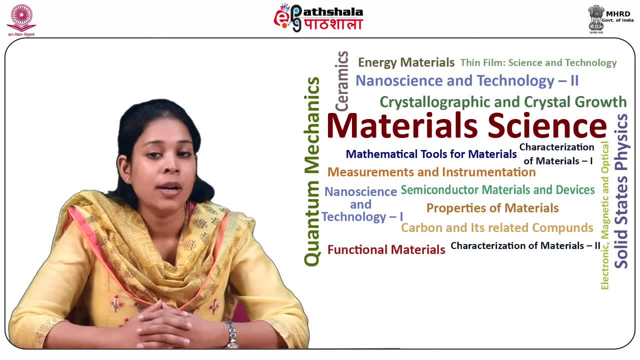 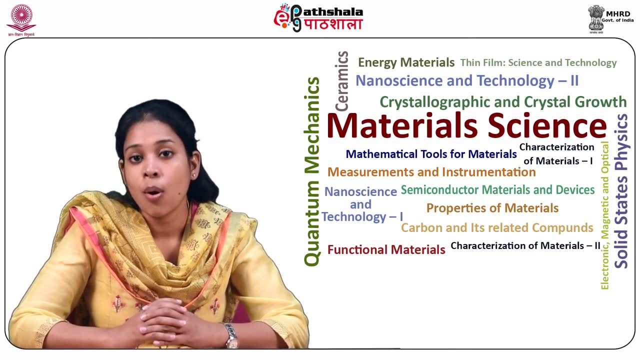 for the formation of elongated grains is more, that is, in the compositions containing ND. So this is because, as the phase stability is low, So the driving force for the nucleation is high and so very few nuclei forms. So in the case of composition denoted by YB1212, that is, M is 1.2 and N is 1.2, which 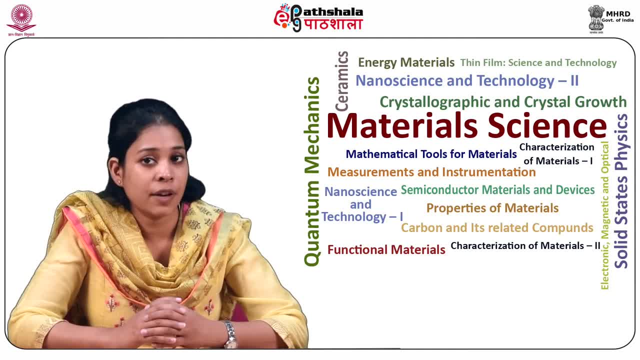 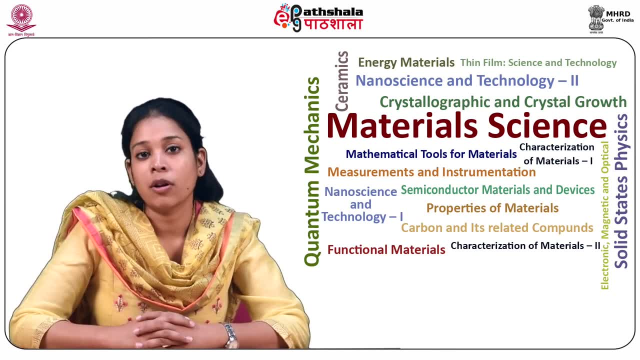 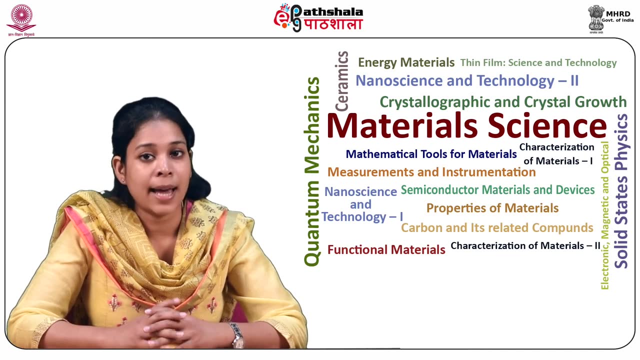 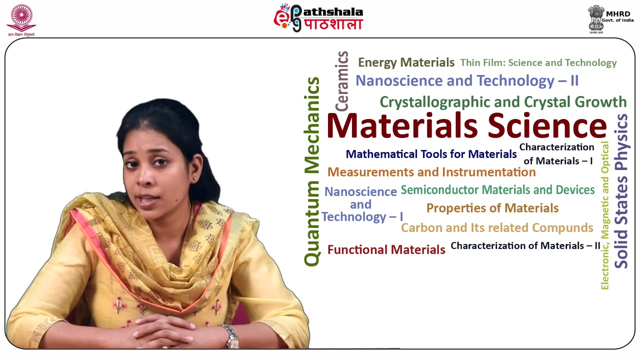 has a very high driving force and a low nucleation rate. A two step process are used for the formation of glass ceramic. So the first is firstly the piece is held at lower temperatures, around 1550 degree Celsius, where the nucleation rate is very low, so that only a few nuclei are. 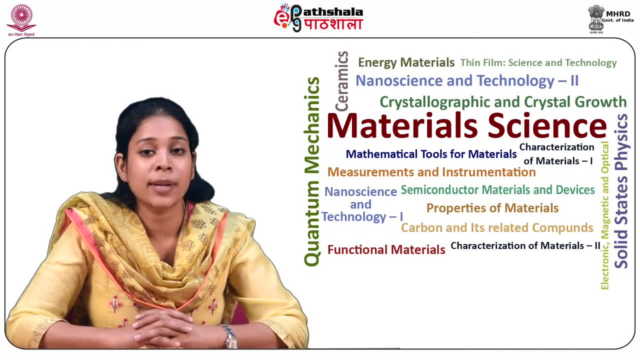 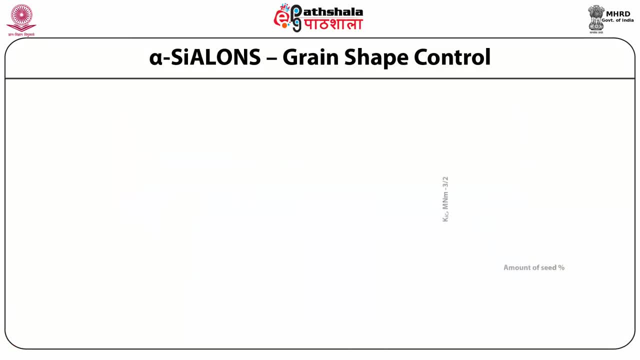 formed. Then the piece is heated to 1950 degree Celsius to form elongated grains from these nuclei. Students, you can see on the left hand side a figure showing the amount of seeds versus fracture toughness for alpha-celon. So, even though it is possible to prepare alpha-celon, 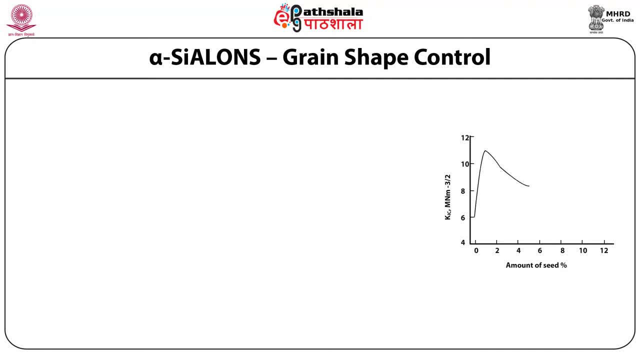 from suitable composition using controlled heat treatment. the dependence of composition, temperature and phase stability on the nucleation rate makes the process difficult to control. An easier alternative is to use seeds of alpha-celons in the starting powders. Thus the alpha-celon is first prepared separately, and then small amounts of the seeds. 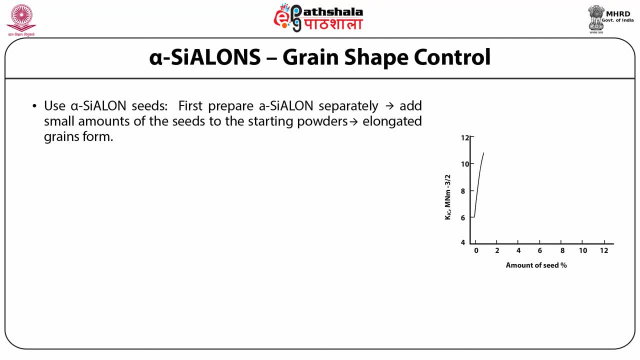 of this are used along with the starting powder. When the amount of seeds is small, the elongated grains of alpha-celon are obtained. ». of the elongated grains, and thus the fracture toughness of the material depends on the amount of seed and can be controlled. So, students, you can see a plot of the amount seed versus the. 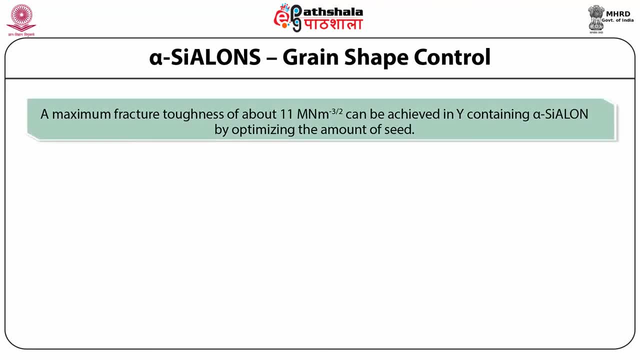 fracture toughness and a maximum fracture toughness of about 11 mega newton per meter to power 3 by 2 can be achieved in Y containing alpha-celon by optimizing the amount of seeds. However, the fracture toughness of the celons is still far below for metals and is inadequate for many. 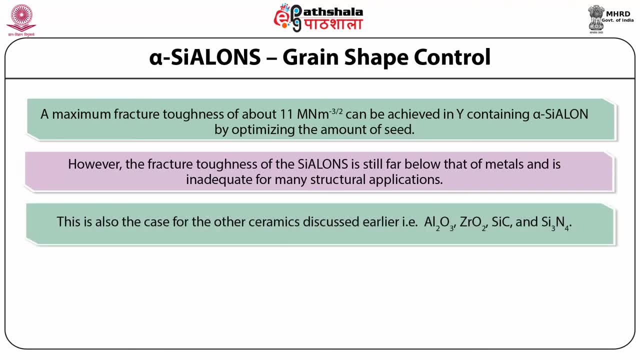 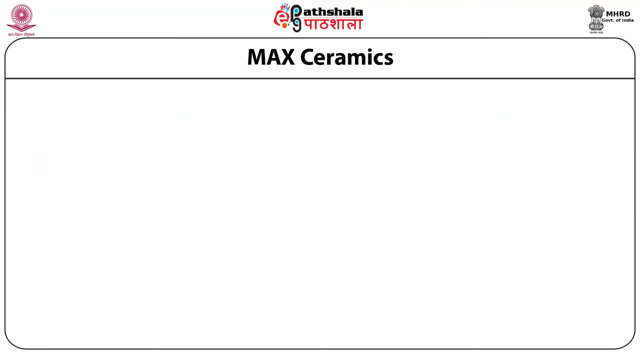 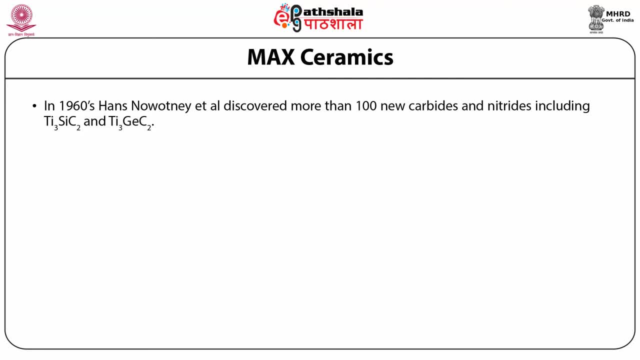 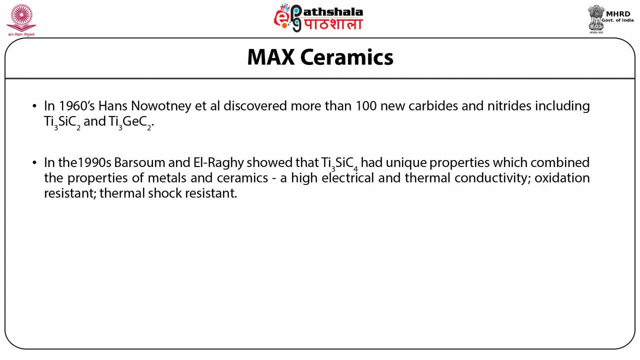 The Balsam and Alpaca were introduced. El Bragghi prepared large samples of Titanium Silicon carbide and showed that it had unique properties which combined the properties of metals and ceramic. Thus it had a high electrical and thermal conductivity like metals and was oxidation. 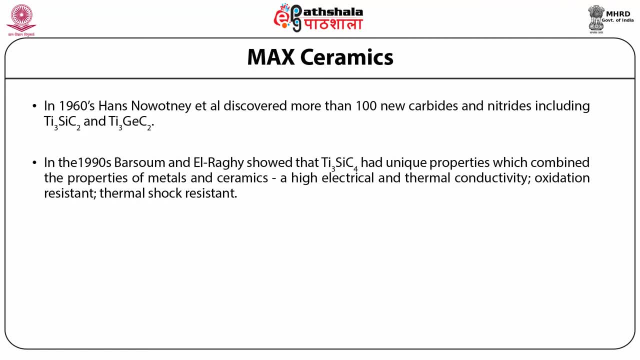 resistance and thermal shock resistance, like ceramics. Later, they discovered that the titanium aluminium nitride, that is Ti-phos GRAMME, was used in the balsam anaerobic lavoro. Later they discovered that the Titanium aluminium nitride, that is Ti-phos GRAMME, was used in the balsam anaerobic�rocrosis and was used in the 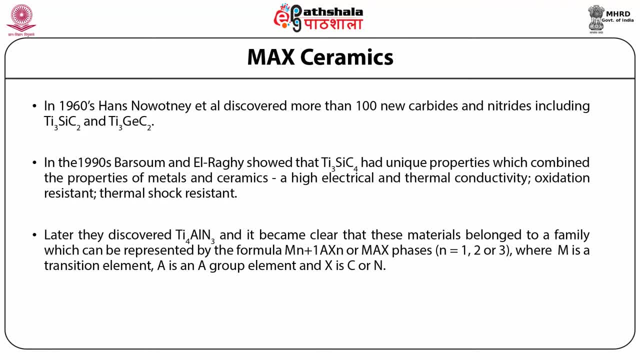 That is Ti4AlN3, and it became clear that these materials belong to a family which can be represented by the formula Mn plus 1, Axn or max phases, where n is equal to 1,, 2 or 3 and m is the transition element, a is a group element and x is carbide or nitrite. 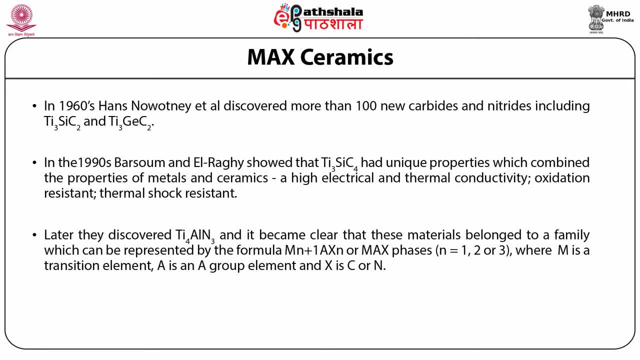 The phases corresponding to n is equal to 1, 2 and 3 are represented by 2, 1, 1, 3, 1, 2 and 4, 1, 3.. The transition element, that is m, can be from group 3, group 4 or group 6.. 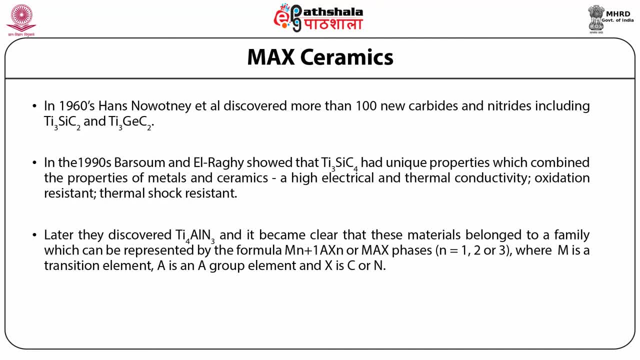 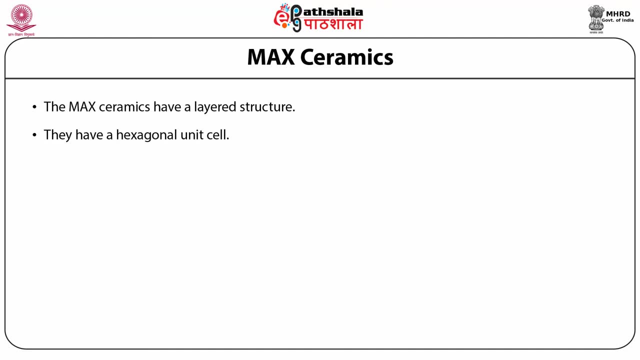 No max phases are known, with the transition elements y or nu from group 3 or w from group 6.. The max ceramics have a layered structure. They have a hexagonal unit cell and there are two formula units per unit cell. The unit cell consists of M6X octahedra with layers. 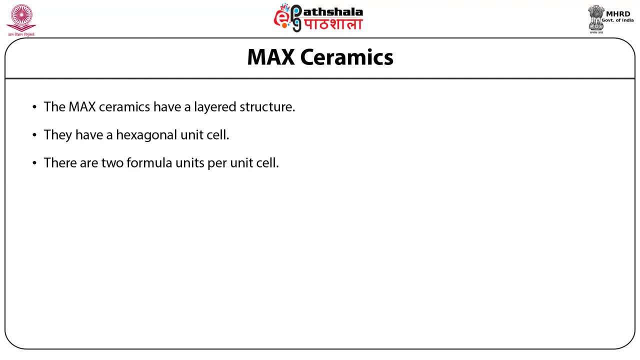 of A element between them. In 2, 1, 1 phase, two M6X layers separated by each other by A layer. Similarly, in 3, 1, 2 and 4, 1, 3 phases, the number of M layers separating per a layer. 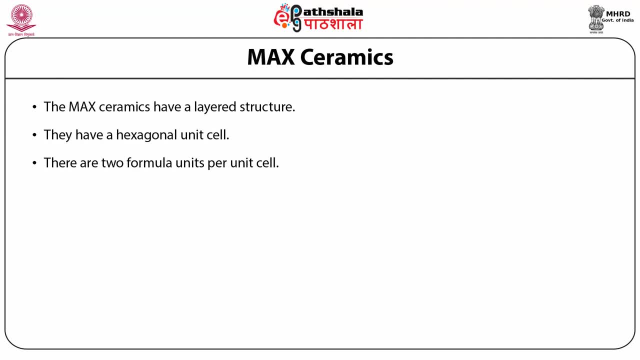 is three and four respectively. In Addition to the pure Max phases, the solid solutions between them also exist. The number of these solid solutions is quite large, and the bonds in the max phases are the combination of Metallic, Covalent and Ionic bond. 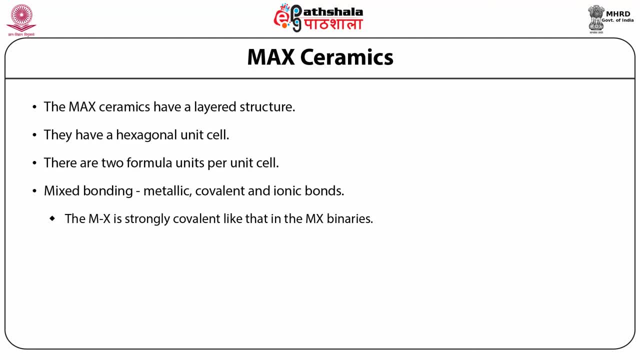 The MX is strongly covalent, like that in the MX binaries, whereas the MD-MD bonding is metallic. Also, the MA bonds are relatively weaker than the MX bonds. The solid solutions between max phases also exist. The number of these solid solutions is quite large. 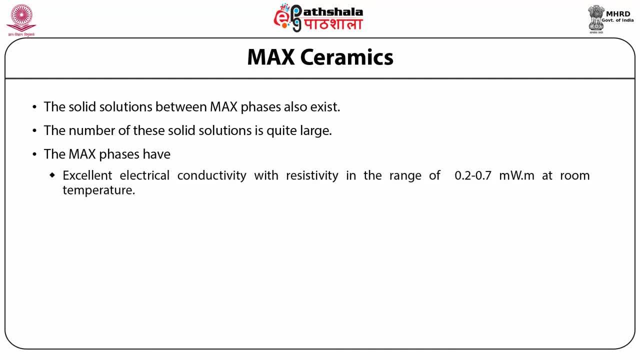 The max phases have excellent electrical conductivity, with resistivity in the range 0.2 to 0.7 micro ohm meter at room temperature. So many of the max phases are so called compensated conductors, in which both electron and holes are the charge carriers. 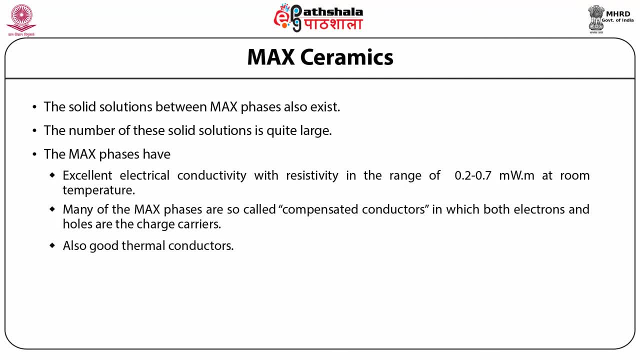 They are also good thermal conductors and their thermal coefficient of expansion They are relatively low, in the range of 5 to 10 micro per Kelvin. Several of them have very low thermoelectric or C-back coefficients. The max phases oxidize in air, but some of them form an oxide which forms a protective oxide layer making them resistant to oxidation. 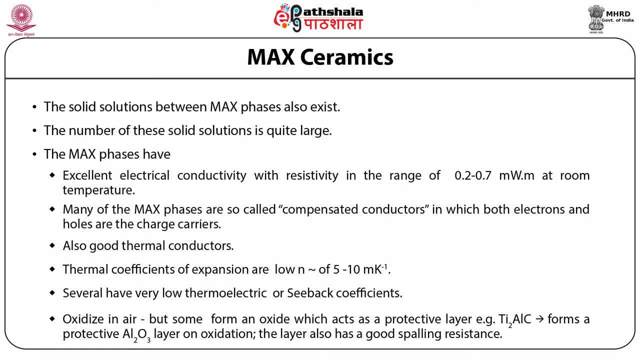 For example, T2ALC, which forms a protective layer. The T2ALC layer is a layer of Al2O3 layer on oxidation. This layer also has a good spelling resistance, making this material quite resistant to oxidation. The max ceramics have near isotropic elastic properties. 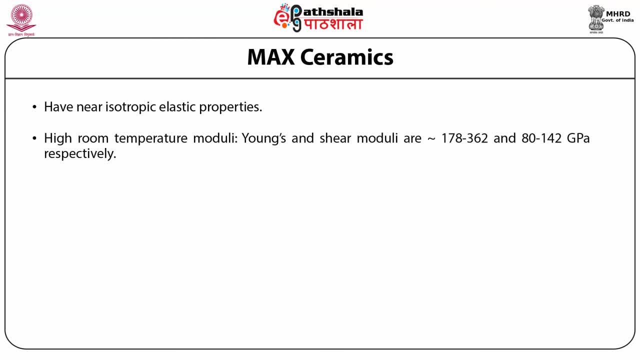 They have high room temperature moduli. ie Young's and Sher moduli are 178 to 362 and 80 to 142.. They also have a very low density, of the order of 4 to 5 gram per centimetre cube. 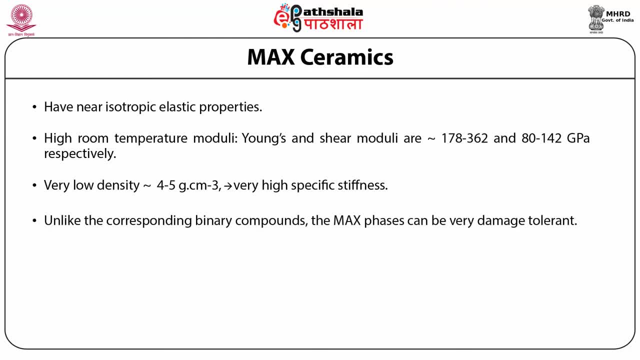 Unlike the corresponding binary compounds, the max phases can be very damage tolerant and therefore, while titanium carbide is brittle, damage tolerant and non-machinable, Whereas titanium silicon carbide is machinable and non-machinable, Whereas titanium silicon carbide is machinable and non-machinable, 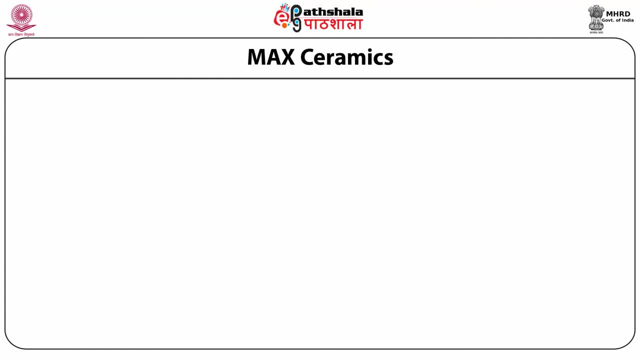 The reason for this is the presence of a high density of mobile dislocation in the max phases. The dislocation are Bessel plane dislocations and, however, since the slip is confined only to the Bessel plane and the number of slips system is less than 5.. 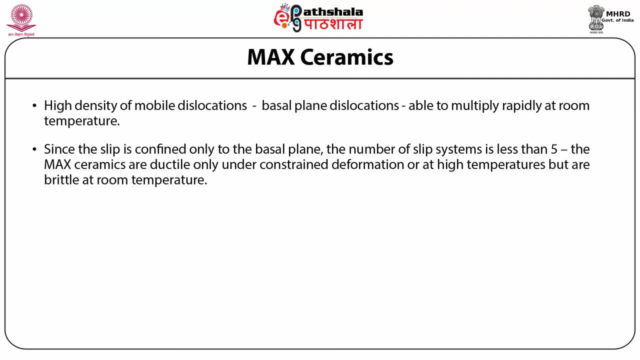 The number needed for good ductability. The result is that the max ceramics Are ductile under constrained deformation or at high temperature, but at brittle at room temperature. Therefore the deformations occur by shear band formation or King formation and by delamination. the max ceramics 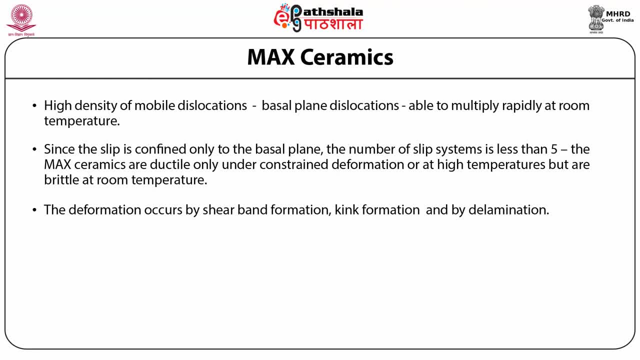 The max ceramics are relatively soft materials. Their room temperature fracture roughness ranges from 5 to 20 mega Newton. In the mid use cases m to power minus 3 by 2. They show an R-curve behavior, the relatively high value of fracture. 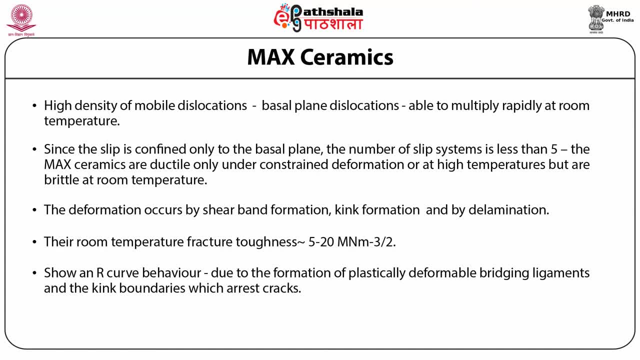 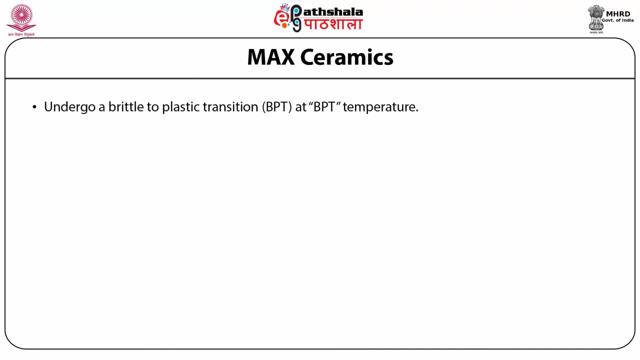 toughness and the R-curve behavior is due to the formation of plastically deformable bridging ligaments and the kink boundaries which arrest the cracks. The max ceramics undergo a brittle to plastic transition status, BPT, at a temperature above which they are quite ductile, even in 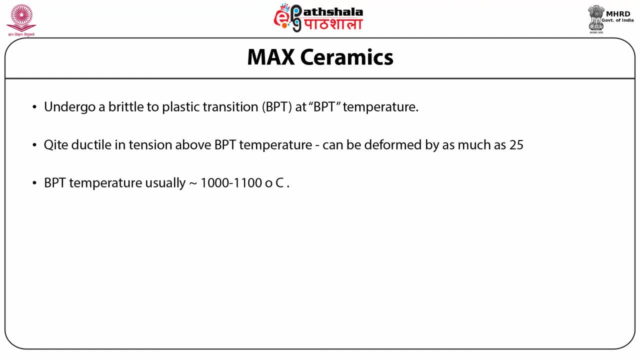 tension. The BPT temperature of any of the max ceramic is found to lie between 1000 to 1100 degree Celsius. They have exceptional resistance to thermal shock and they do not shatter or quenching from high temperatures Easily. they are machinable by conventional high speed tool. 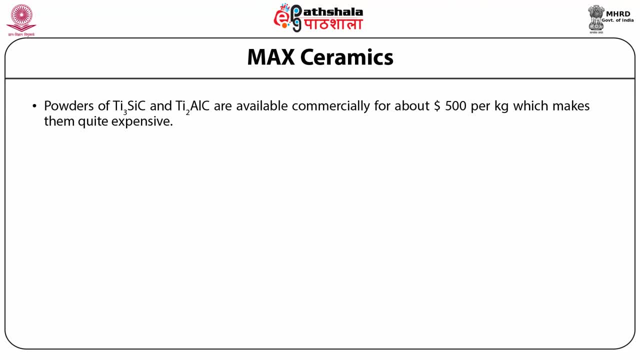 and the powders of titanium silicon carbide and titanium aluminium carbide are available commercially for about $500 per kg, which make them quite expensive. They can be sintered in pressureless manner to high density and, despite of its high cost, the ability to do 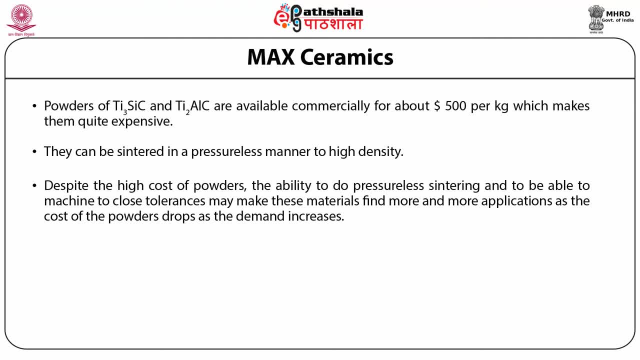 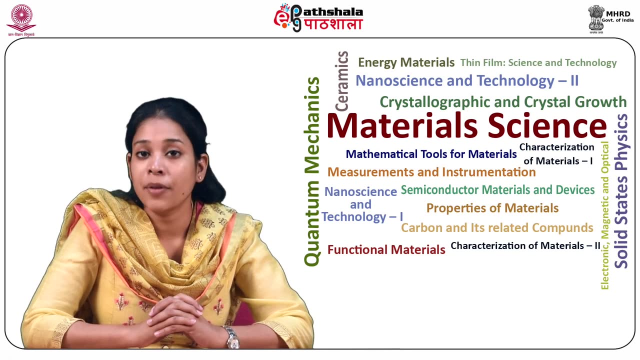 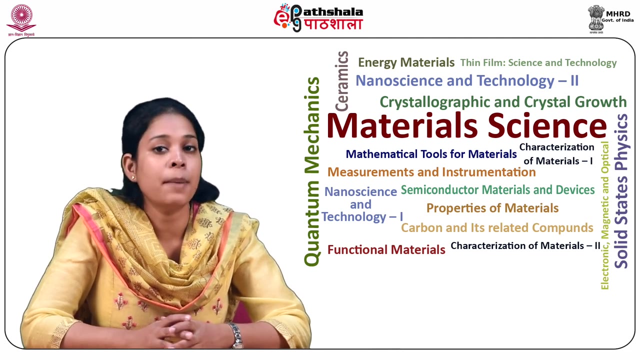 pressureless sintering and to be able to machine to close tolerance may make these materials fine. So, students, let us summarize what we have learned in this module. So so far, we have learned that the room temperature fracture roughness is around 5 to 20 mega Newton m. 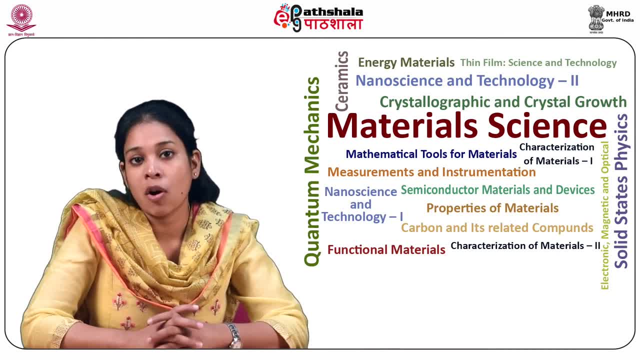 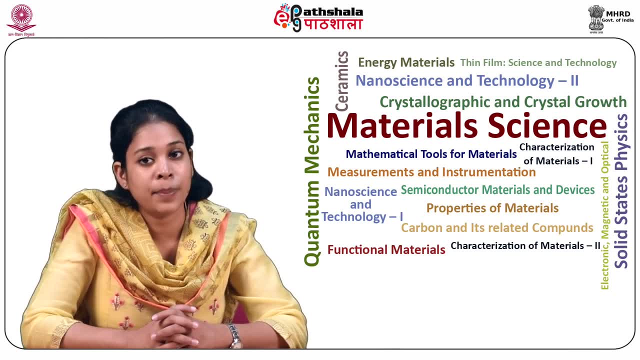 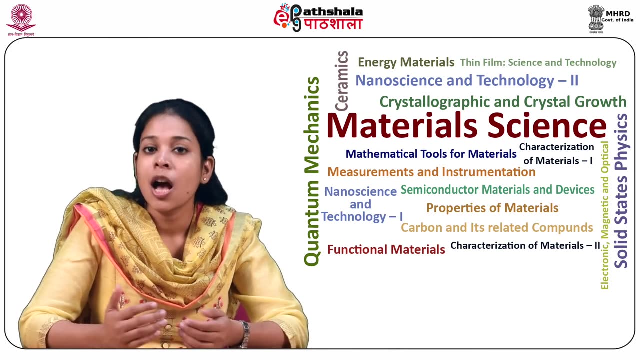 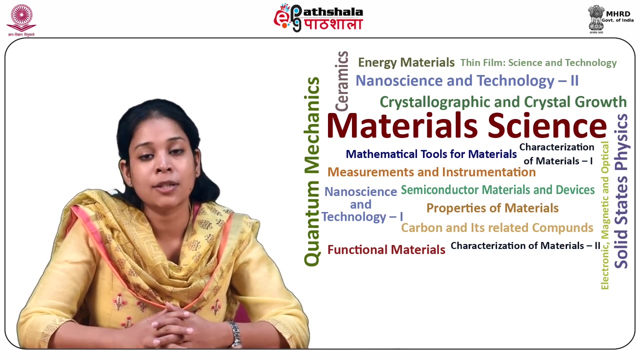 to power minus 3 by 2, which can be seen from R-curve behavior. It undergoes a brittle to plastic transition status- BPT- at BPT temperature and it is quite ductile in tension above BPT temperature and can be formed by various method as much as 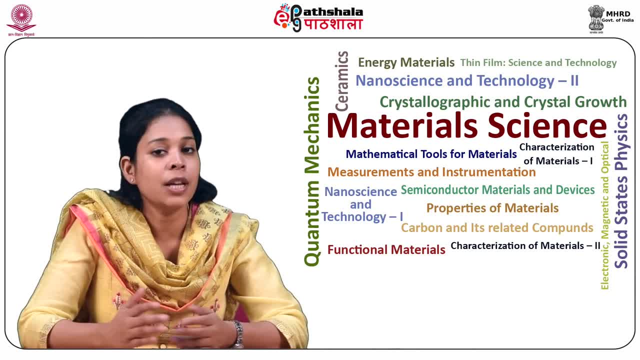 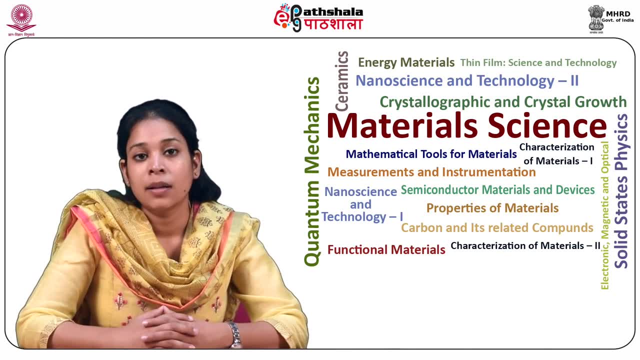 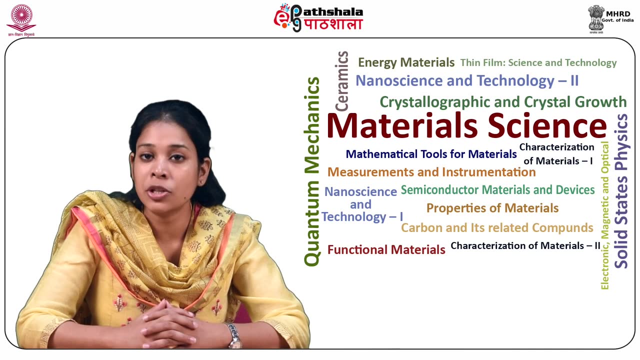 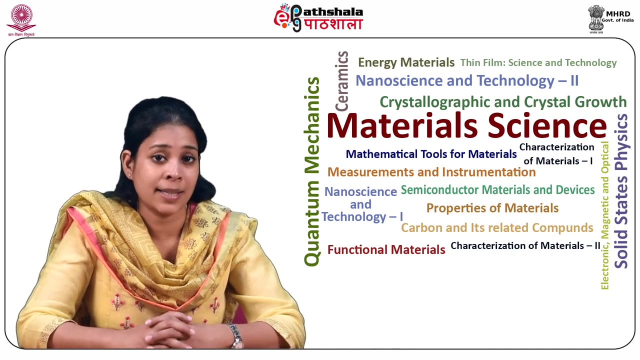 25. So BPT temperature usually varies in the range of 1000 to 1100 degree Celsius. They have an exceptional resistance to thermal shock and do not shatter on quenching from high temperatures. Moreover, they are easily machinable by conventional high speed tools, and primarily because of